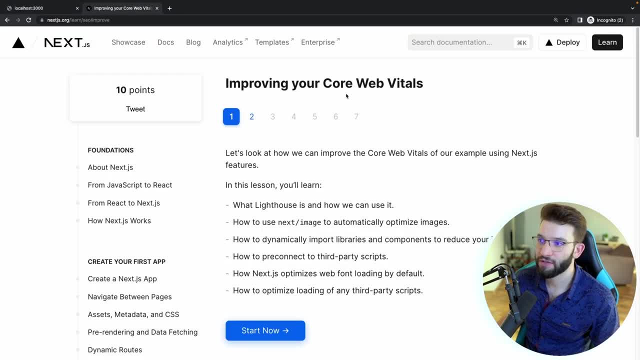 actually following the best practices from the Nextjs website on like the core vitals or core web vitals. They have actually a lot of advices in here and instructions on how you can do that from like oh, how you can test it in Lighthouse, how you can use Nextimage to optimize images. 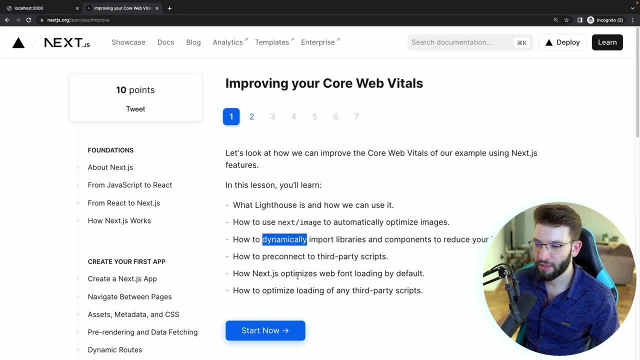 dynamically import libraries, pre-connect like third-party libraries, funds optimization, loading third-party scripts and so much more. I actually used this and added a lot of more stuff to actually improve it to its best. So, before we get started, we have a really, really awesome. 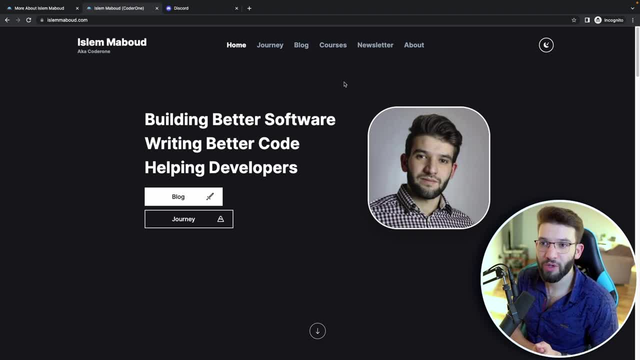 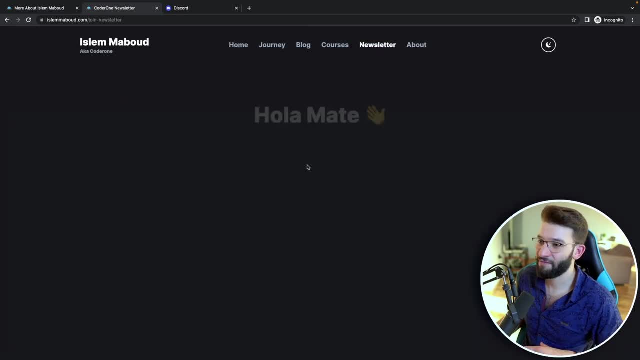 and also how you can use Nextjs, and also how you can use Nextjs, and also how you can use Nextjs. What we're also going to have in here is a really awesome newsletter that's going to have a lot of developers and you can actually join us. We have like a b-weekly newsletter specifically made for 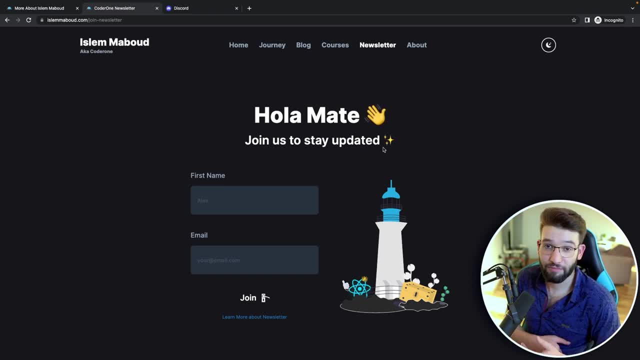 developers for like finding out new jobs, maybe like knowing about new courses we're going to be releasing really, really soon. You can learn more like blogs and so many stuff in tech in here- how to learn the jobs in a perfect way. So you can make sure to go ahead and join the newsletter. 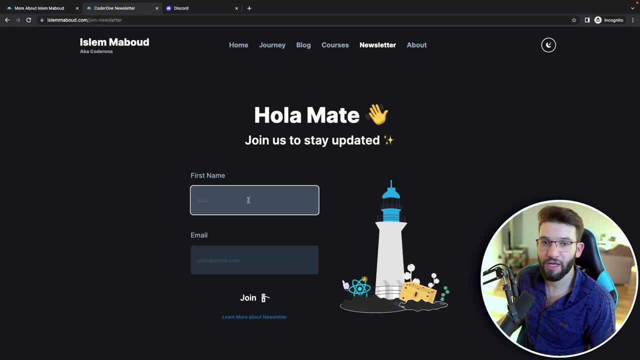 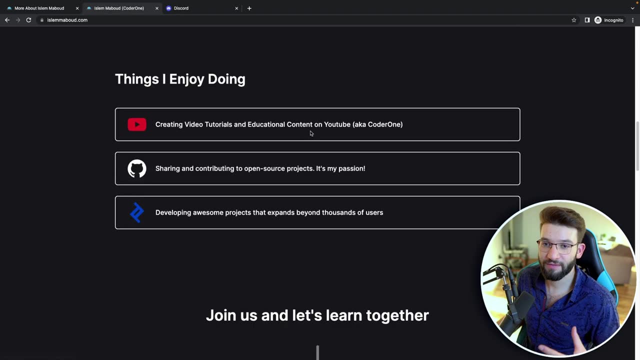 on islamabootcom: forward slash. join newsletter in here. Put your name, your email and you can email and stay tuned for a b-weekly newsletter, As well as if you ever want to join in our discord and share thoughts, need help or you want to basically collaborate with other people. 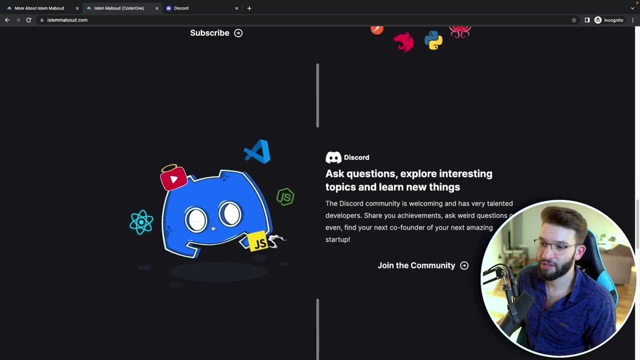 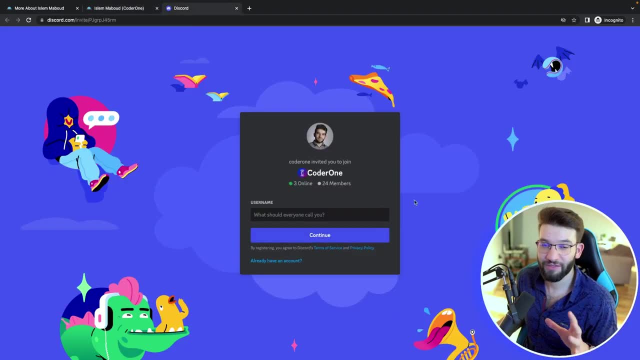 I have a lot of resources over there. You can just go down in here and actually find the discord here or just click on join community. It's going to take you right in discord server in here You can continue and you can actually just join us to have a bigger and a better community, Also before. 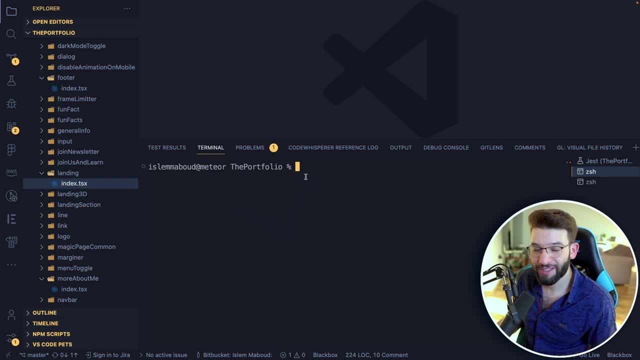 we get started in here. actually the way to run a production build of Nextjs on your local host without actually deploying it So you can always test on Lighthouse on a production build, It's actually by doing yarn build. So make sure yarn build is going to run and actually build for you. 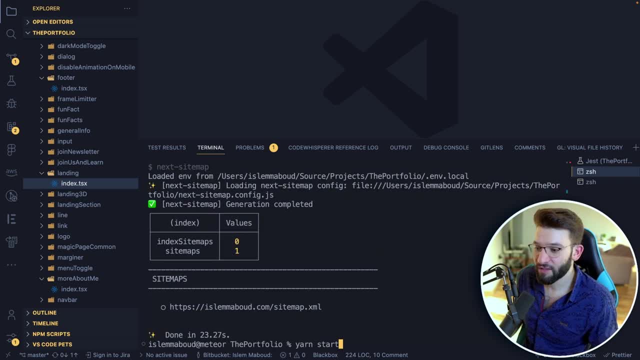 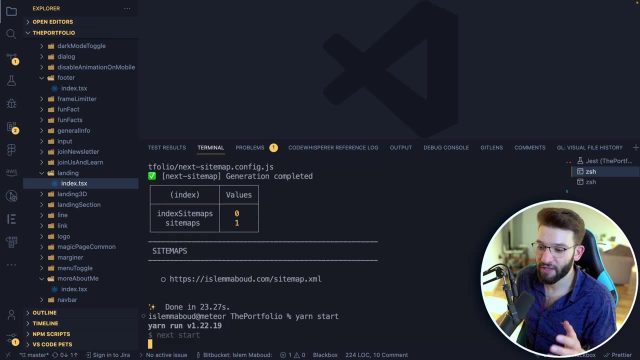 a production ready kind of build And after that one is done, you can basically run yarn start in here, which is going to start the server like a production ready server using the build that you just run and it's going to put it by default on port 3000.. So this way you can run Lighthouse. 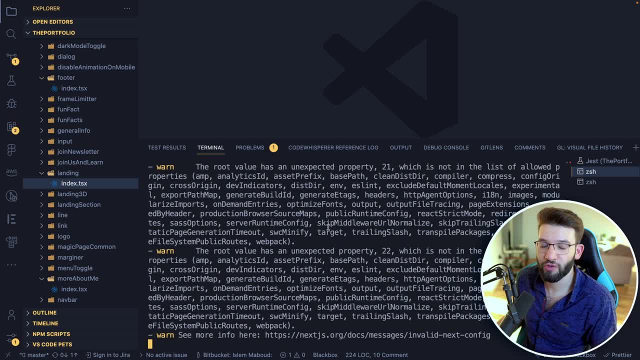 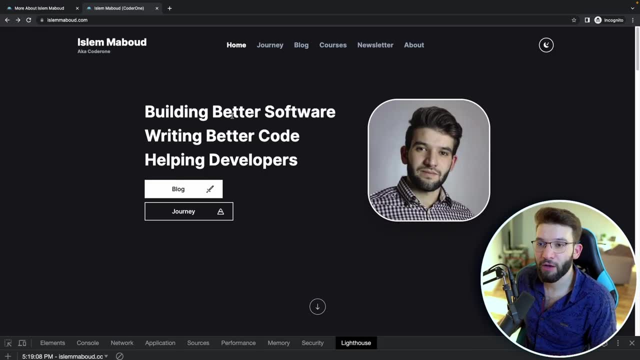 which you always should: run your Lighthouse on a production build. You'll never want to actually run it on a production build. It's going to give you a very horrible kind of scores. Also one other thing in here: before running Lighthouse, what you want to actually make sure you do in your 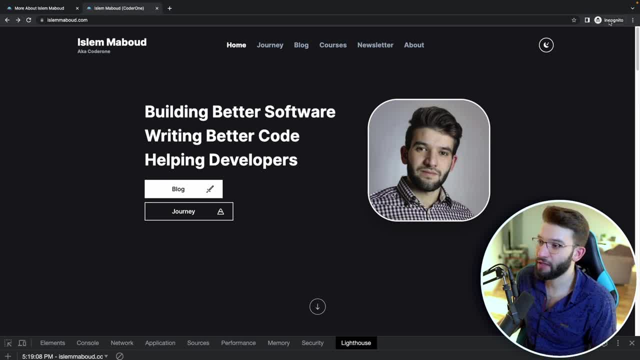 browser, for example using Chrome in here. So you always want to make sure you run it on incognito and you want to run it without no extensions, because running like Lighthouse with extension sometimes it bugs. sometimes extensions actually have a very huge bad impact on the score itself. 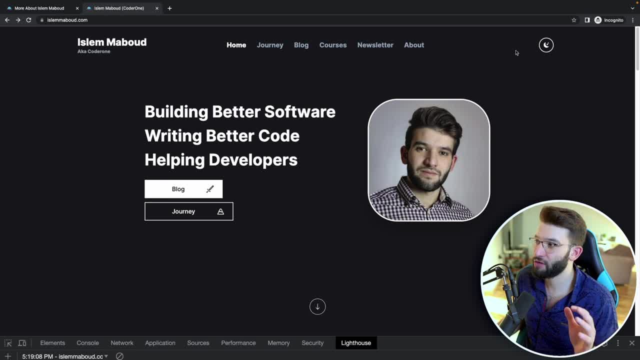 because they load some third party stuff and whatever. So you're always, always, always, always want to make sure you're running on incognito mode in here And you have all the expense extensions basically disabled, All right. So the first step we want to 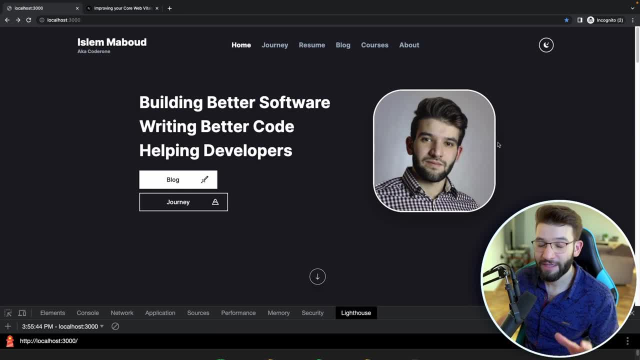 actually optimize, and what we're going to do is actually optimize images, And, yes, images. it plays a major, major role of any website, because nowadays, like websites, can't you know, you can't have a website without having a decent set of images, and they're all that high resolution. 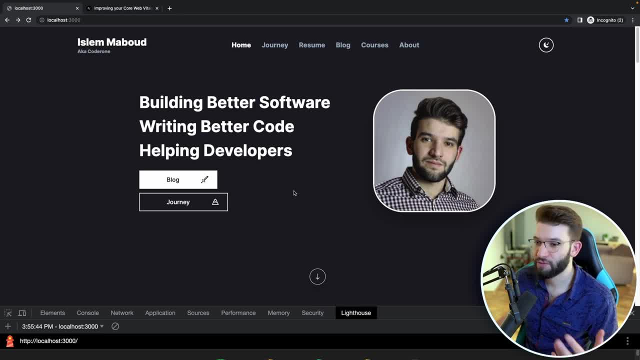 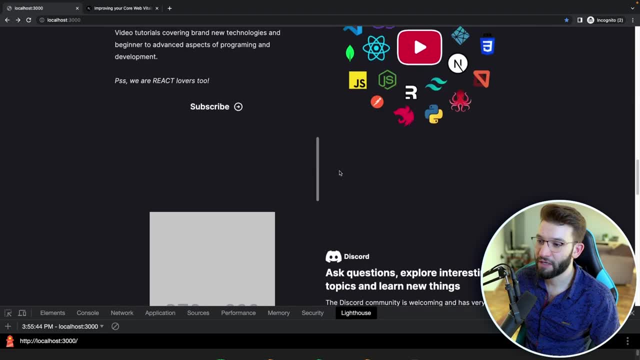 They're very large in size, They have a lot of constraints and responsiveness and stuff like that, So you have to basically optimize them to its best. So, for example, in here I've got like a couple of images. Um, I have like 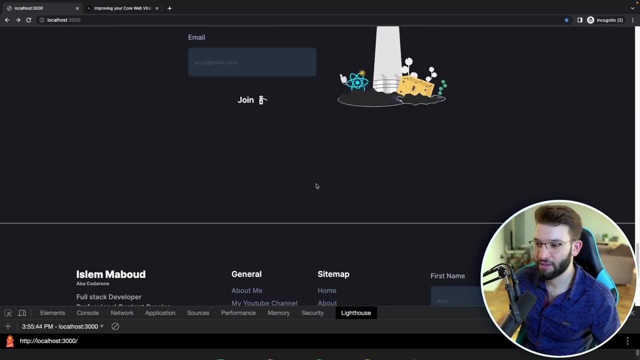 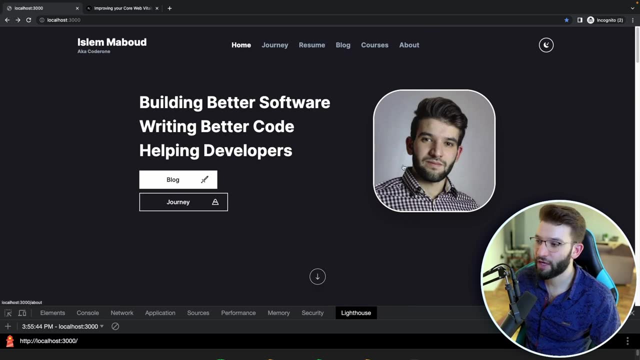 maybe this one in here. this one is a placeholder. I replaced it in upcoming ones, but maybe like this, this one is an SVG, but let's say I want to optimize this image, my portfolio kind of image in here. So if I look into the Lighthouse in here, they did run And remember this is actually the. 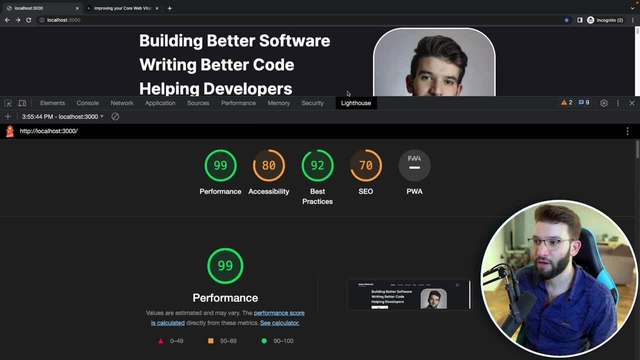 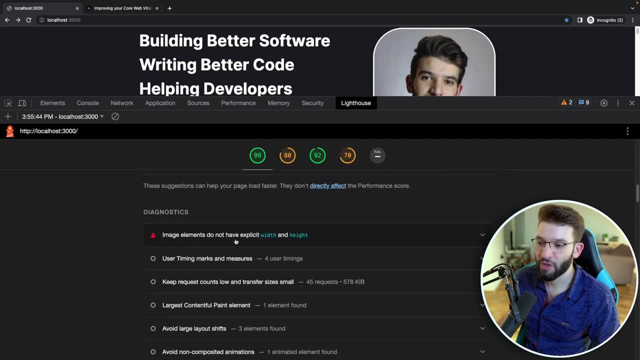 bad one. So we are in like kind of like the non optimized version of the website. So in Lighthouse in here, if you look into it and just scroll down a little bit in here, I've got in here like image element. do not have an explicit width and height, So it maybe just kind of complains. 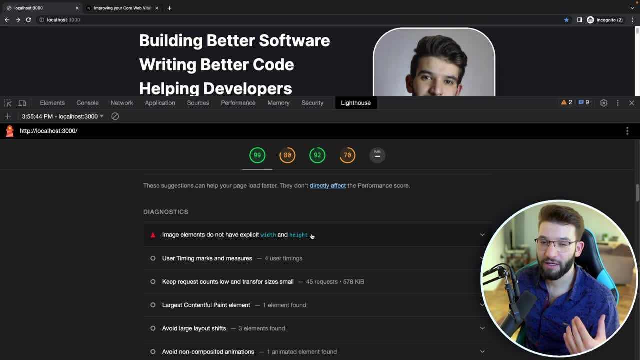 the width and height, because sending those explicitly kind of kind of like helps you kind of avoid uh UI shifts or just shifting the UI in the CSS when the website is being loaded. So what Lighthouse in is actually recommends we go ahead and use the next image And yes, 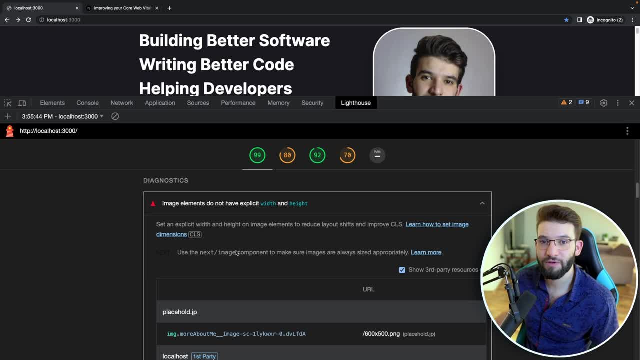 this is actually correct. So you basically want to use always. if you use it next years, you want to utilize this really, really awesome component, which is called the next image which has been released since, like the version 13,. I guess something, And this will just basically. 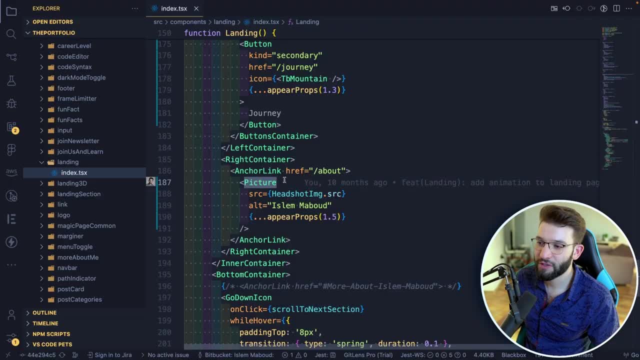 give you a lot of stuff. So inside of the counter, what I'm going to do in here is, for example, this picture in here is our picture. So if I try to go ahead and see the definition, I'm using stock components in here And for the picture. 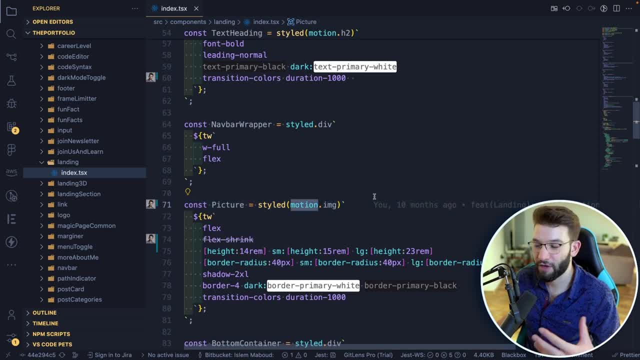 I'm using motion dot image, which is just basically using frame emotion for animation, And this is just simply the HTML image. So technically, I'm not actually utilizing or not using the next image custom component. So you can do in here is go ahead and use the image. 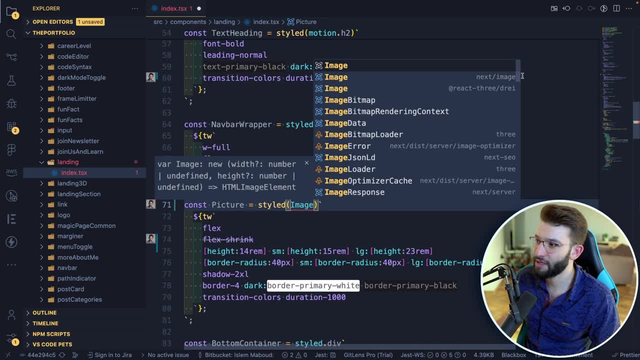 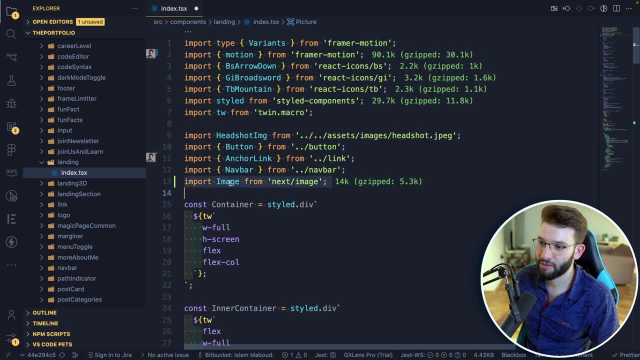 component So you can just make sure you select that. actually import this from. next image is increasing on the top in here So I can click on it. It's going to automatically be imported for us using VS code. But if you don't know that, that's actually basically being imported from where? 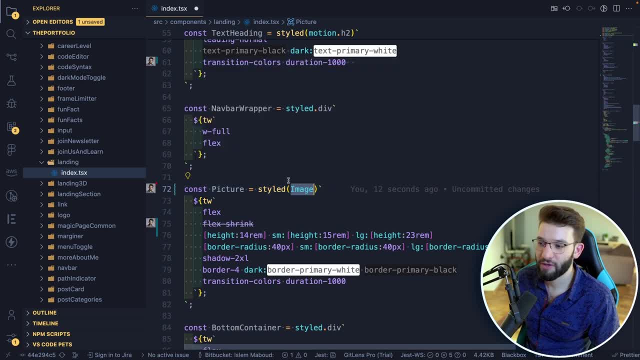 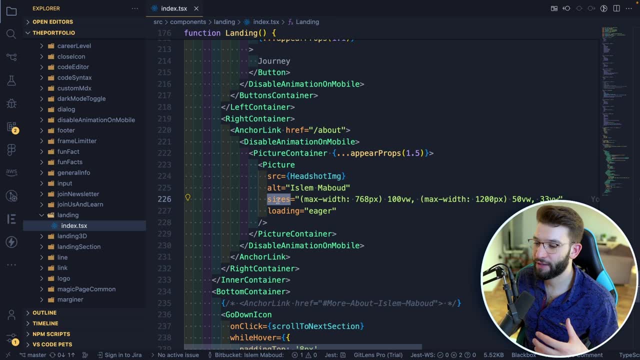 and these will just technically will well, was to basically work with images better. So now we can actually use the sizes property, which is a very, very important one when it comes to the next GS image components, And it kind of like helps a lot optimizing your website. 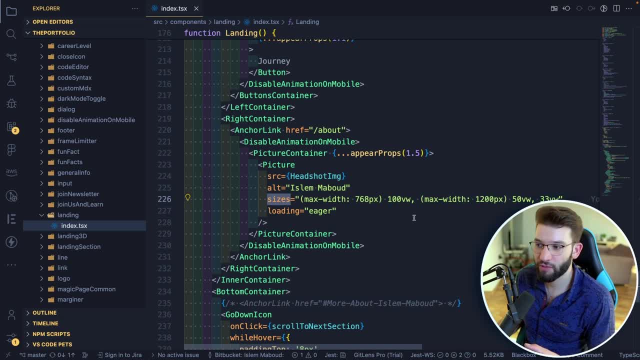 and helping it like: load faster depending on the screen size- So the sizes in here, basically what it tells it- you can actually load responsive images. So you say, Oh, if the maximum width is seven, 68, which is more of like a mobile kind of. 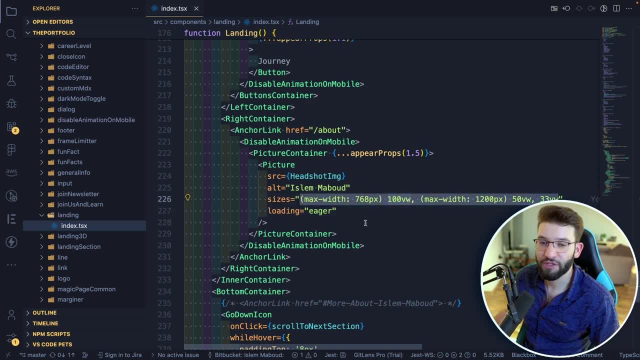 tablet view. So I want to load like the whole image by itself, So like the whole size of the image, a hundred viewport or view within here, sorry, And maximum within here, for example, for like laptops. I want to just only hold like a, like a portion, like a 50% of it. 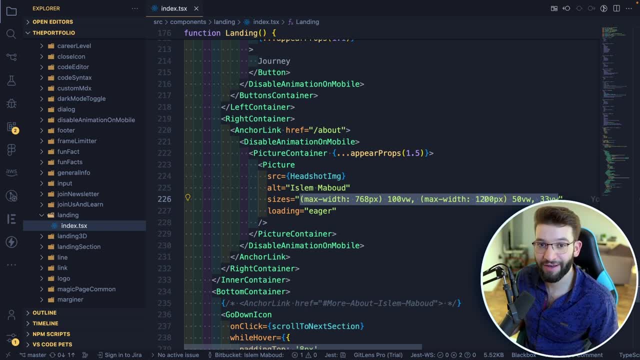 So you can imagine if it like a 50%, which can decrease the size of the image, and behind the scenes everything magically happens and being generated for you. So technically, next year is behind the scenes going to take those stuff in here that you put in here and the different sizes. 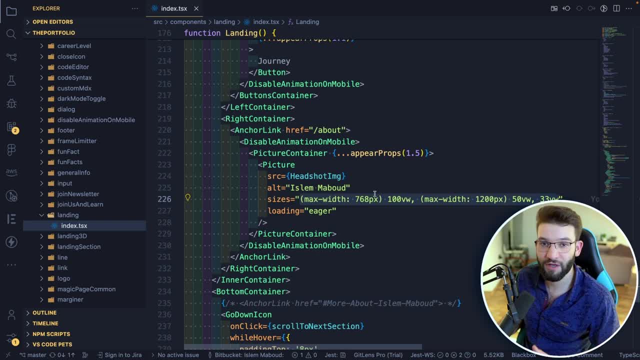 you put in here, it's going to generate for you. So you can see that you can load different images depending on the sizes you put, and this will help your website load a lot, lot faster, because it depends on the images And as soon as the images 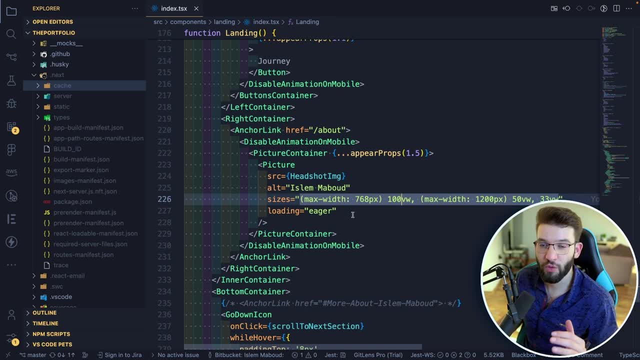 are becoming visible. it just going to be a lot better And it's going to score better in lighthouse And, of course, here for loading. you always, always want to set this to eager. You'd never want to do it for laziness, unless you have a really good reason to. but most of 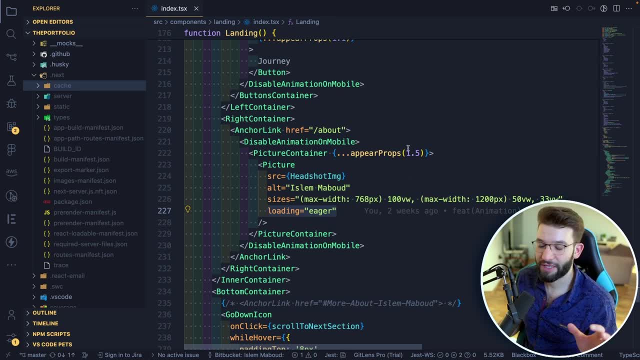 the times you don't want to actually do that. Eager loading is the best for image because kind of just like loaded as soon as the website or the webpage is being loaded. it's going to make it a lot faster. It's going to like crease the score in your lighthouse. The other important part for 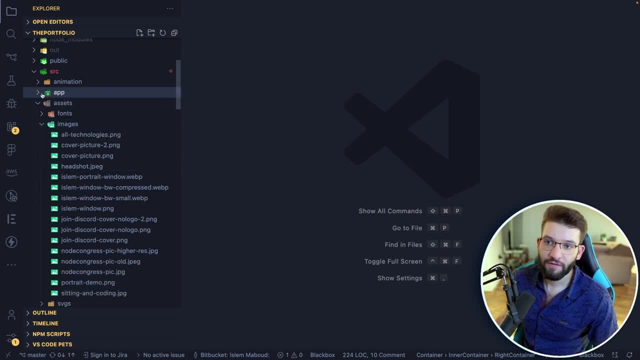 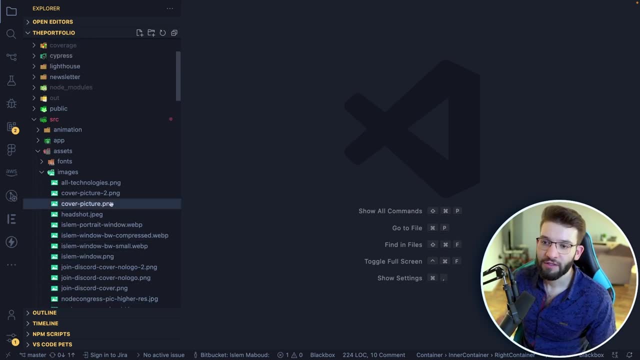 image is actually compressing images. So for example, in here, for instance, if I go inside of my like assets folder, I have a bunch of images like pictures of me- uh, maybe, you know, going to a conference, stuff like that. So for example, here I got this picture where it's: 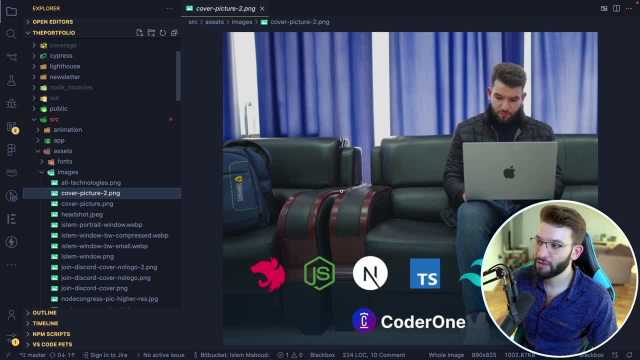 actually like a cover picture, So I have two sizes of it. So cover picture two, which is a very large one, is actually the first one before I did resize and compress that one. So it was like 990 pixels And it was like a one megabyte. That was ridiculous size for an image. So what I had to go through is actually: 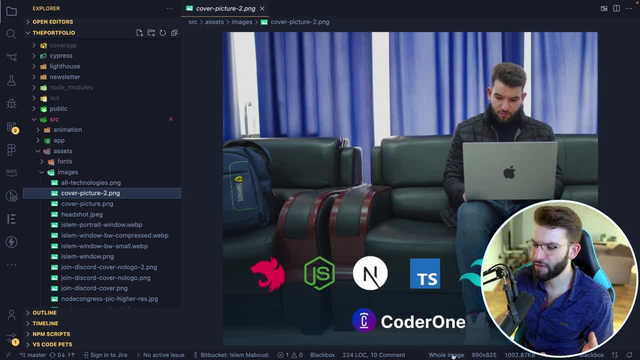 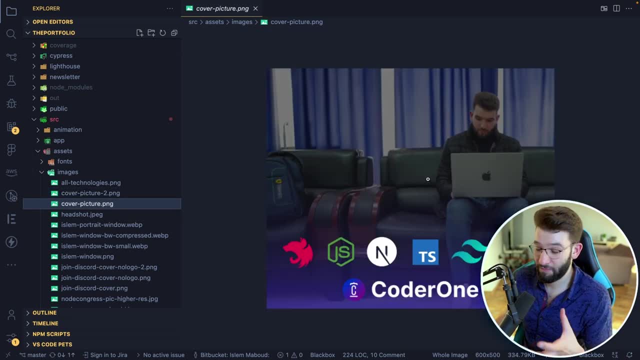 compress the image and resize it, because I don't need that huge size, I don't need this 990 pixels in here, So simply, all I need is more of like just 600 pixels, and it just can fit that perfectly. And it did resize this from like one megabyte to 334 kilobytes. The second thing you want to. 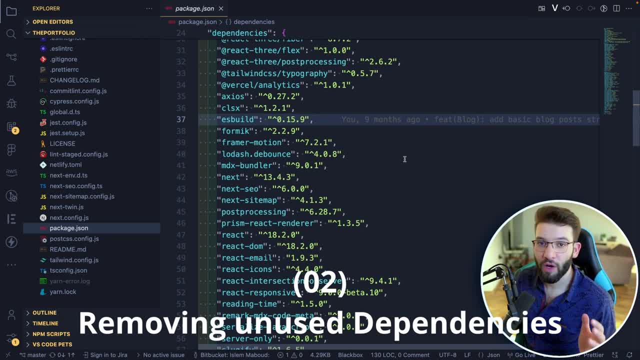 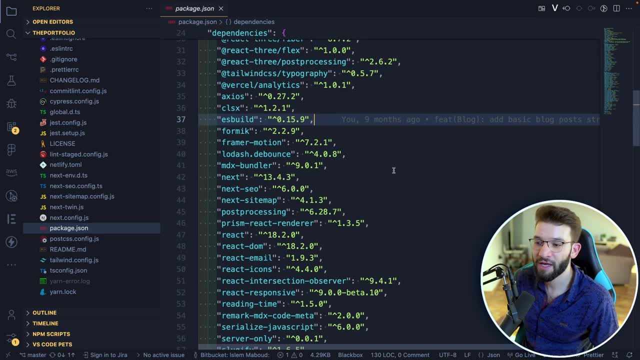 actually make sure you do is removing unnecessary or unused dependencies, because, as as developers, we tend to install our dependencies And we just like completely forget about them over time And those dependents actually gets somehow into the latest bundle, which is going to make it a lot bigger, And it doesn't actually need to. 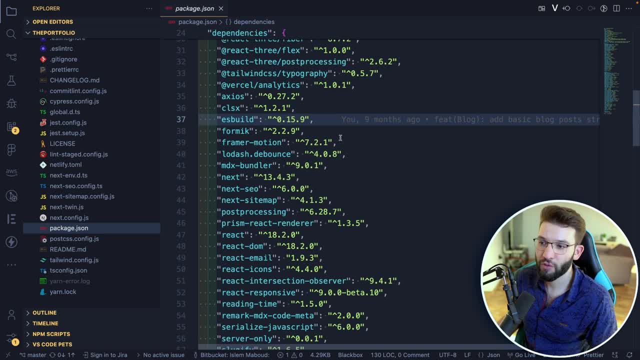 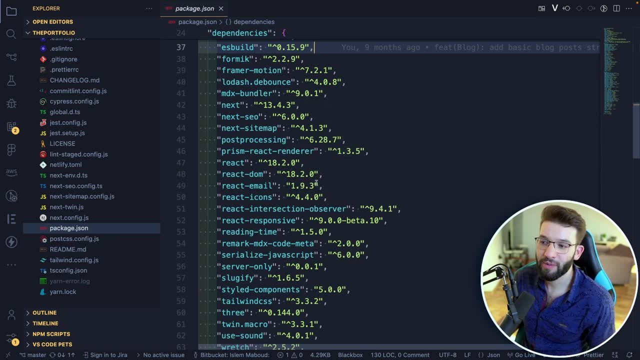 be because you don't need those dependencies in the first place. So simply make sure you just go through all your package or JSON dependencies in here and try to inspect what you're actually using and what you're not using inside of your code. Or maybe sometimes you're using a very large one. 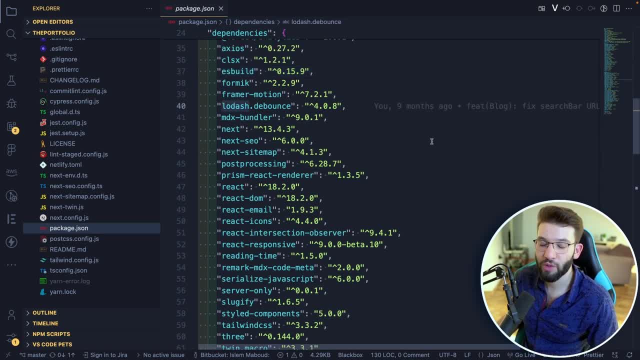 for example, in here I've got like this example for like low dash- And we all know that the low dash library has a lot of utility functions- And, of course, installing low dash and actually loading all the utility functions and sometimes you're only using one or two of them, It's just 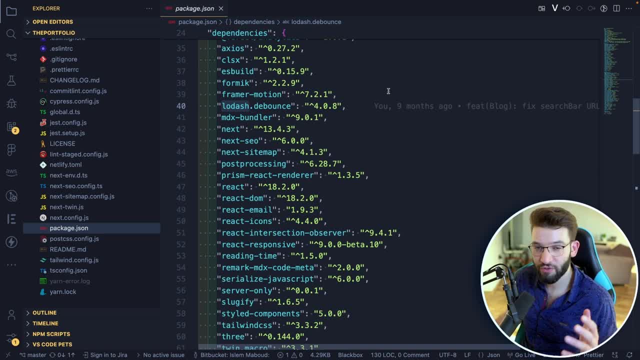 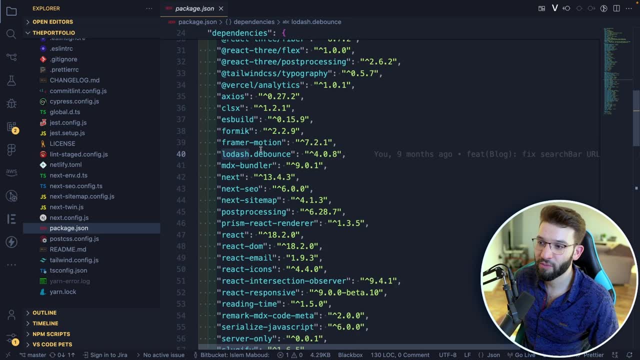 insane. It's going to make your bundle size explode, even though tree shaking- and some of you guys say, oh, tree shaking and next GS- actually works. Yes, but not always perfectly. So what I tend to do in here. for example, I only needed the debounce function from low dash, So we went. 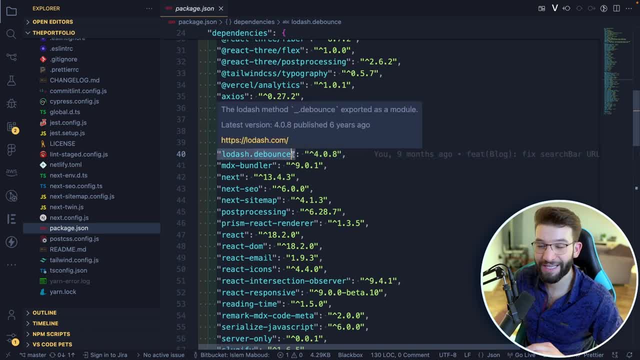 through and actually installed only the low dash dot debounce, which is just gonna install me a one, and always make sure to double check and see what dependencies you have and what dependencies you need to remove because they already did like prune or remove some of the unused dependencies in here. 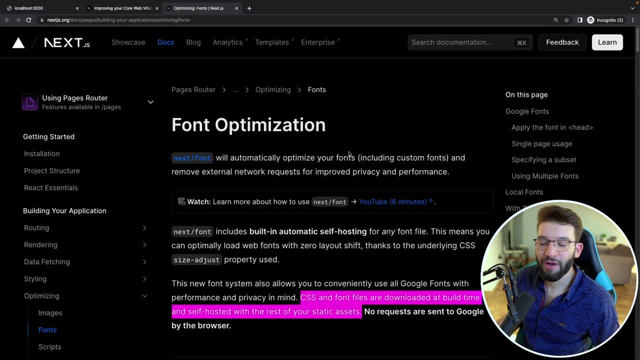 The third step is actually fund optimization. Yes, you're hearing it right- actually loading funds. And if you're basically loading more than one funds out of your website and if you're, for example, loading from Google, you're doing a huge mistake, because in next GS it has a really, really awesome. 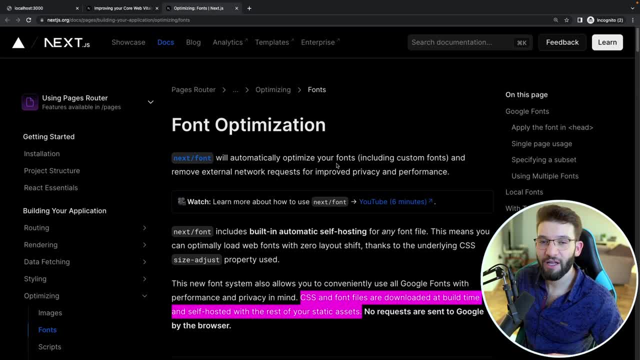 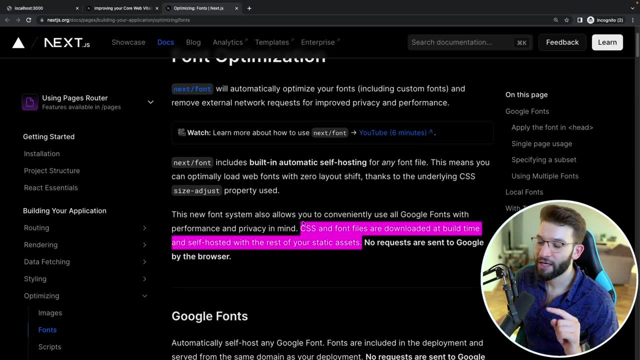 built in package called next for slash funds that actually allows you to automatically, kind of like, do everything for you. It's just super magical. So, for example, in here, what it actually allows you to do, actually download the CSS and fun files are gonna be downloaded at build time and self hosted with. 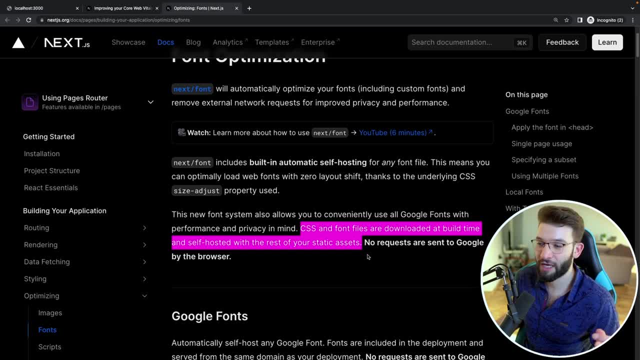 the rest of your static assets by next GS. So all you gotta do is just tell it which funds you want to have- For example, you wanna like use enter and other kind of funds from like Google funds- and it's gonna do the rest for you And, yes, it supports Google funds. in here You can use Google. 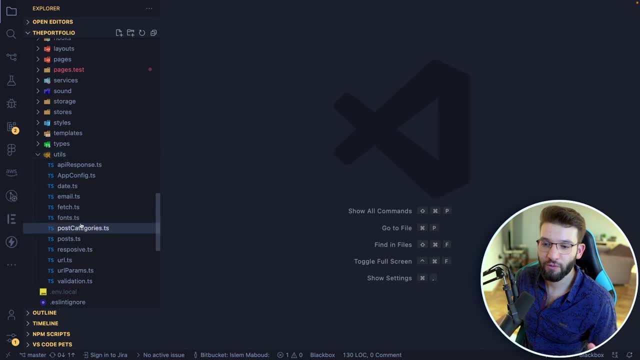 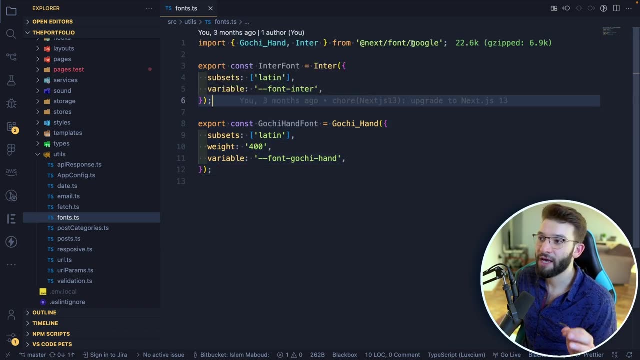 funds however you want. So for example, what I did in here go through like utils folder in here I created a funds dot TypeScript file, actually export all the funds. that actually set up all the funds inside of in here And I'm using 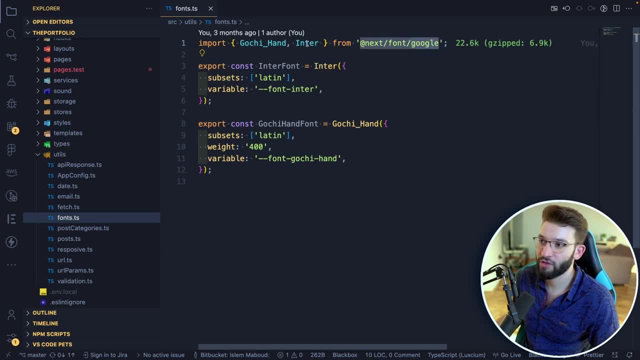 all of those from the next fund package. So access like the Google package in here. So I load this to Google funds and actually tell it, like, what is the variables and stuff like that, For example, the subsets in here. oh, if you wanna use Latin and stuff like that, and same thing in here. 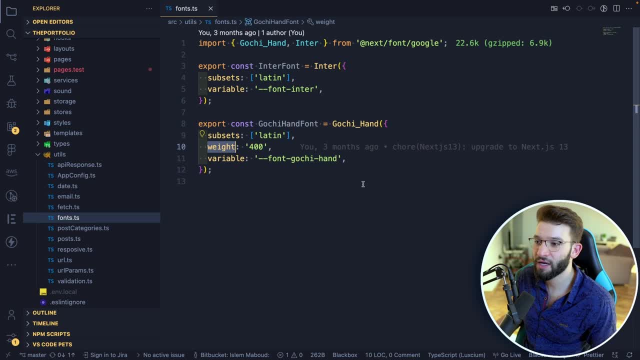 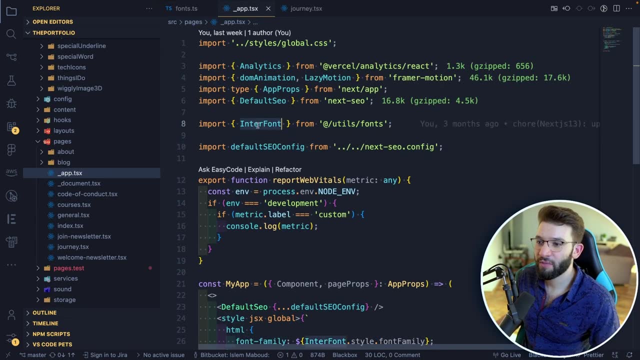 for example: oh, you wanna only load a single weight, or you wanna load all the weights in here. So you can do a lot of customization and tell it which funds should be downloaded and cached for future use, And you can easily use them later on by just doing enter funds in here, For example. 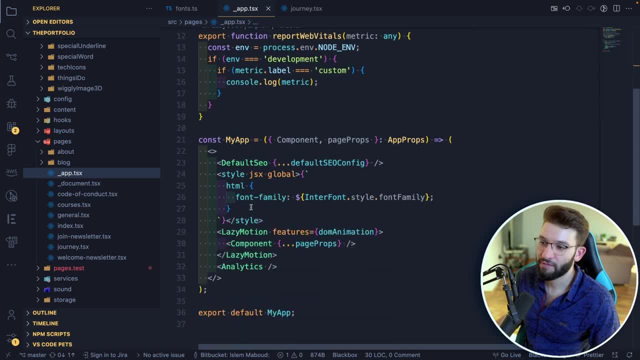 according to the fund that you already created from you know. next funds in here, for example, you just set: oh, you go inside of the HTML, you set the fund family into the funds in here and just the fund family and everything's gonna be generated for you. The fourth one is: you wanna? 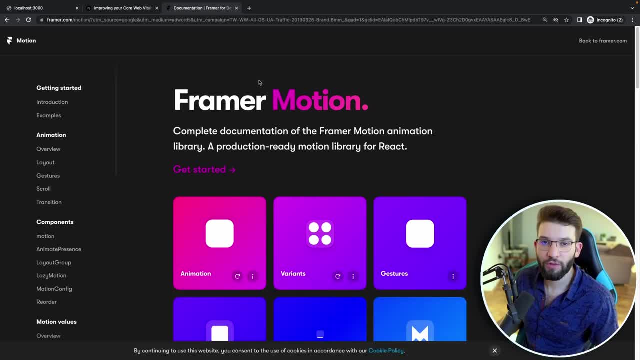 actually go through and actually disable animations, particularly only on mobile. Of course this is just like an edge case, but like 90% of the time is disabled animation on mobile, It's gonna improve the overall user experience and the load time of your website. 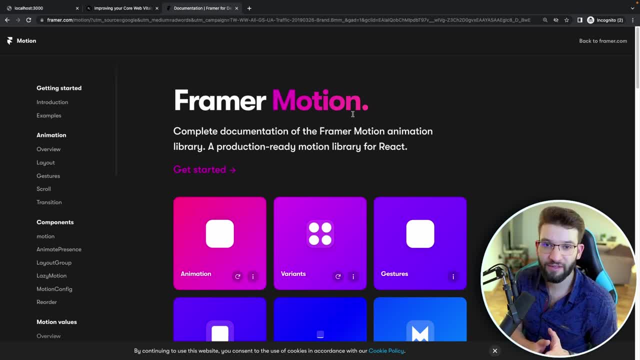 because, as we all know, mobile devices are like a user accessing like your website through their mobile, through like 3G or very bad networks. Most of the times, they're not gonna have the ability to load all this animation actually wait for them, And sometimes it's super laggy, as they have the experience in my website. 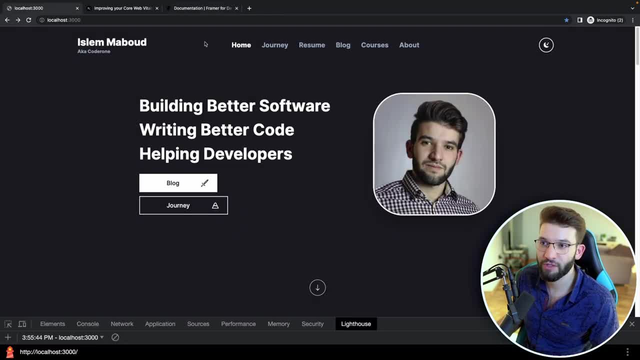 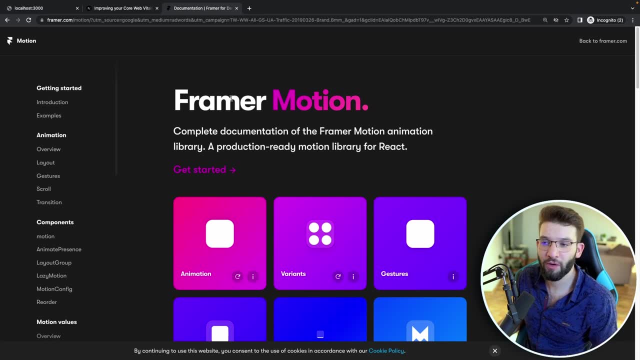 in here. the animations on mobile were super, super laggy using frame of motion. So what I had to go through and do? actually frame of motion in here only disabled on on mobile. So disable completely the animation on mobile. So check if it's mobile, disable the animation. 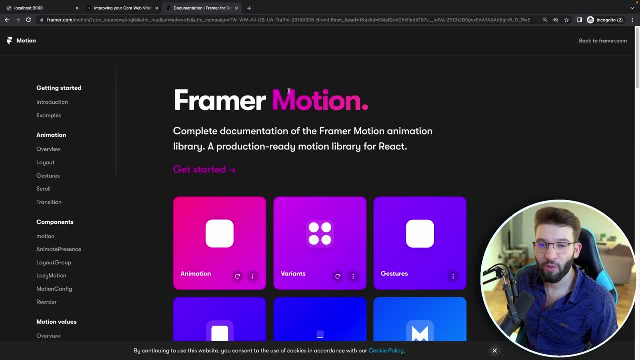 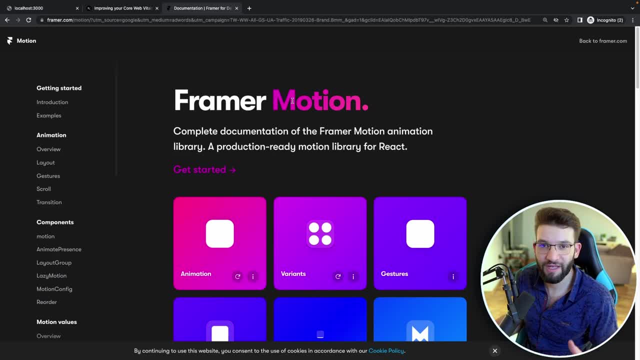 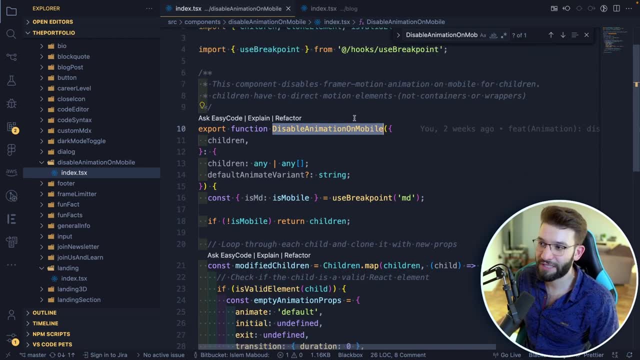 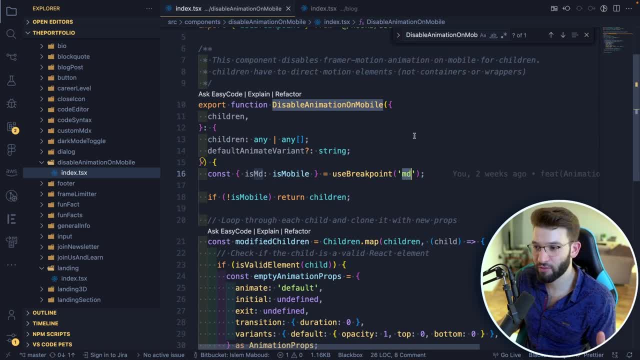 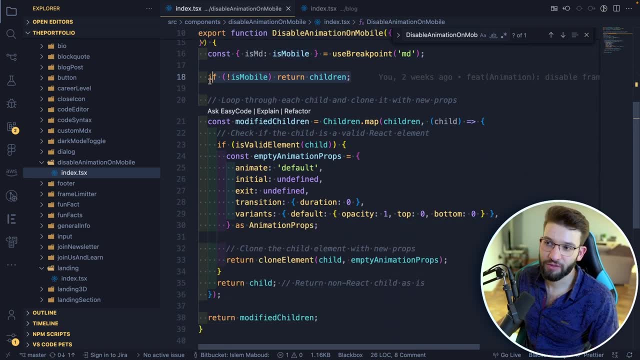 which is like 767 in width and pixels. So that means we are in mobile And if we own, moving on here, I just simply go ahead like returning this: If you're not on mobile, just do nothing, But if you're on remove out, just go ahead and clone the children. 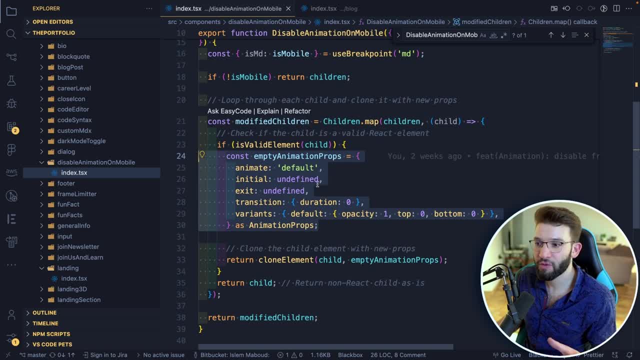 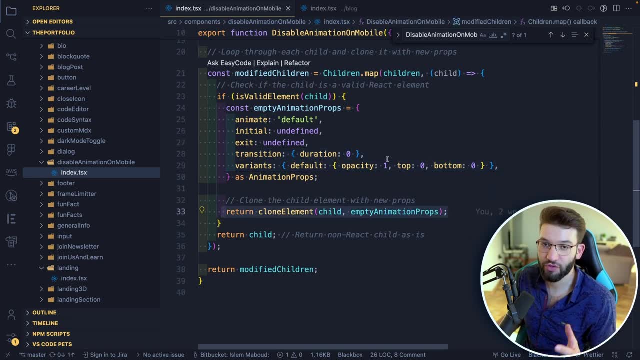 in here and modify the props, which is, you know, the, the frame of motion props in here to disable animation and make them like a default props in here to completely disable everything and just clone the elements and return it. and of course, later on, for example, inside of my blog, here, the 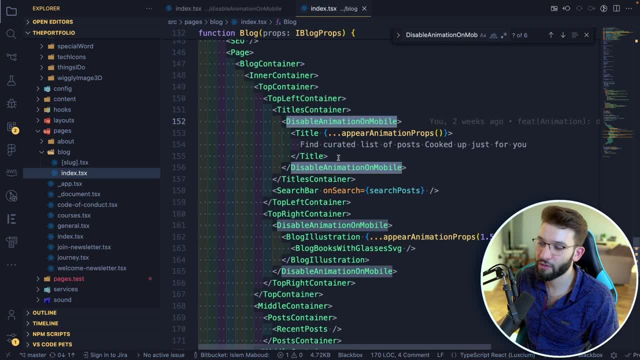 blog in here usually has this really awesome appear animation in here on the top, but simply in here, i completely disable that using this on mobile. so this: actually, if it's desktop or if it's higher than md in width, it's going to work perfectly, but if it's actually less than md or 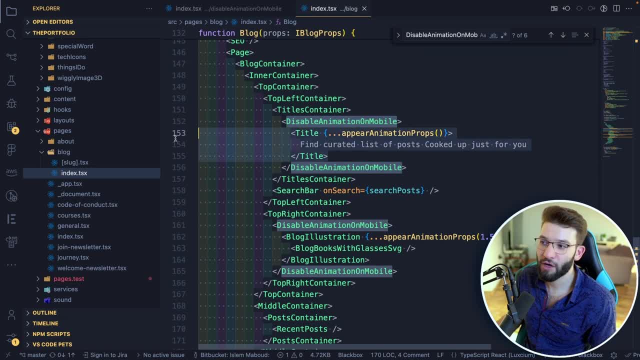 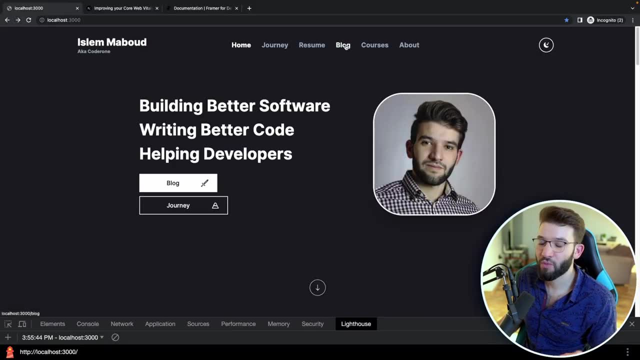 equals to md, that means it's actually in mobile and that's completely going to overwrite. you know, all the props is going to be returned by this function and it's going to completely disable animations. so, for example, if we try to look into the website in here, we are in desktop and if you 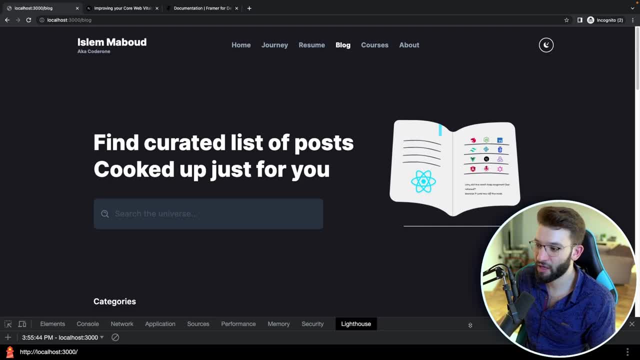 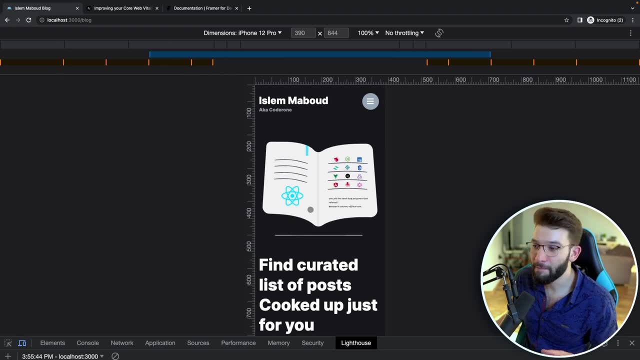 click on it. as you see, the animation works perfectly on, basically, desktop, but if we try that on mobile in here, i'm just using responsive mobile in here and try to refresh the page on the blog. as you see, it appears immediately, without any intermediate editing, which is going to make it feel faster, for, you know, slow networks and mobile users. the fifth: 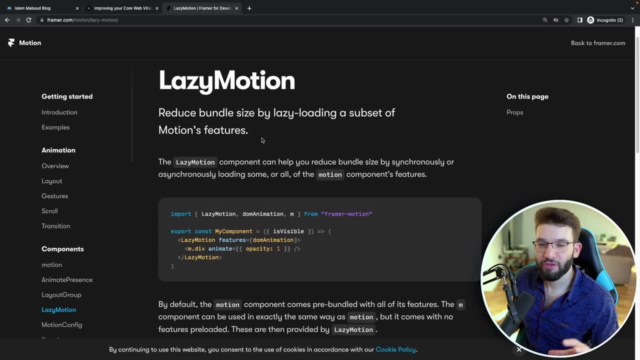 step that you can actually do in here if you're using frame of motion. i'm not sure about other animation libraries, but for frame of motion you can actually reduce the bundle size by quite a lot by just using this lazy motion component. so lazy motion in here is going to tell basically frame. 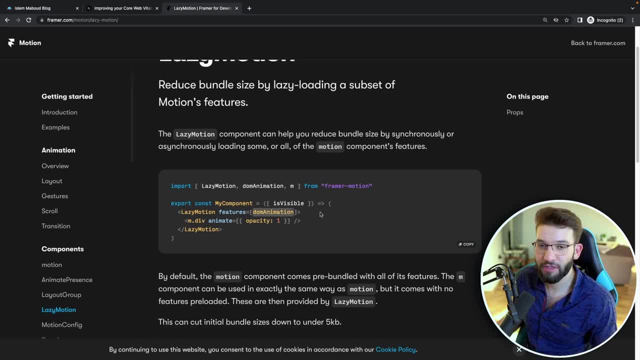 of motion in here that you don't want the full animation capabilities from the library. you don't want to import everything at once, but instead you want to lazy import them, or you can only just provide exactly what you want. for example, in here you only want to just do dom animations and not all the type. 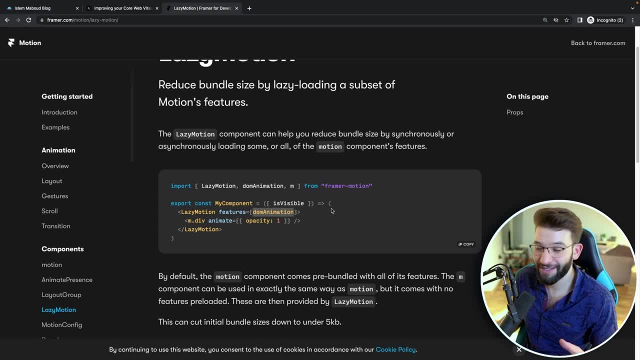 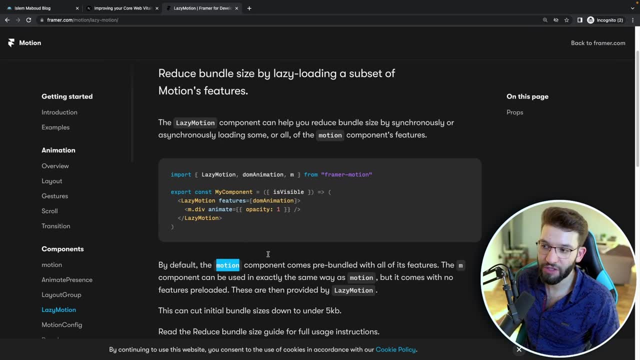 of animations in here like gestures and stuff like that, and that's going to cut the kind of, like you know, bundle size by quite a lot. and of course you can replace the motion library in here which, or basically the motion import that you import from frame of motion through, with this like m kind of. 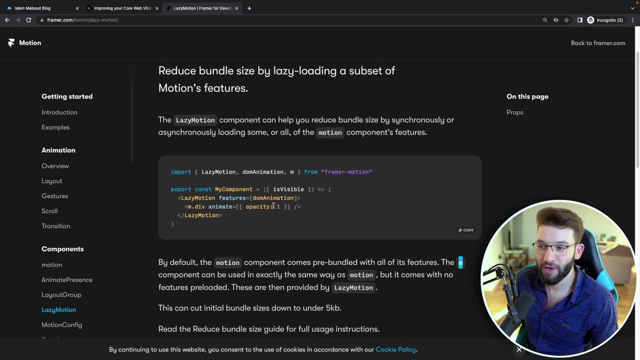 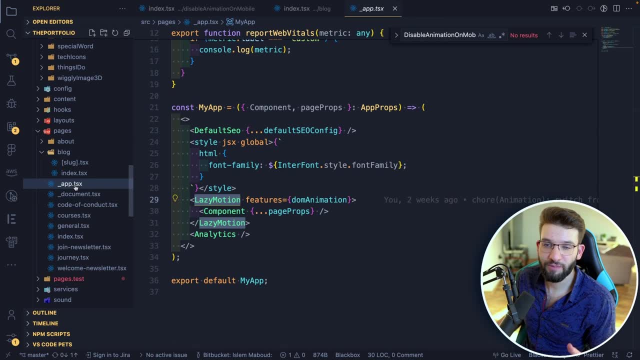 like import in here, which is like a lot smaller, a lot lightweight, and it only uses the you know lazy motion kind of loaded stuff in here. so for example, in here for the library and what i'm using it, i go the up dot tsx in here where everything starts rendering so the roots and i put this lazy motion. 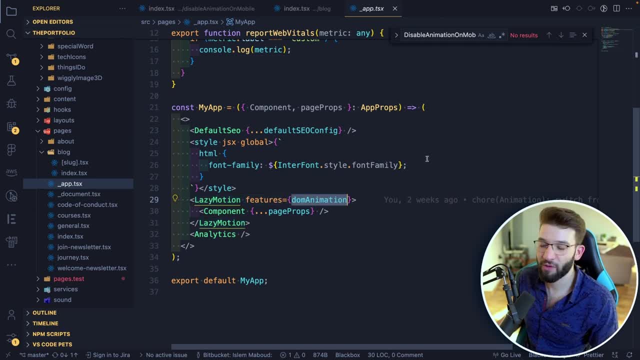 kind of component. and of course it did tell it which features i want, and for now i only want dom animations, because all i'm doing just some opacity, color changes and some transitions. i'm not doing any complicated gestures or drag and drop or any of that's very complicated stuff. so 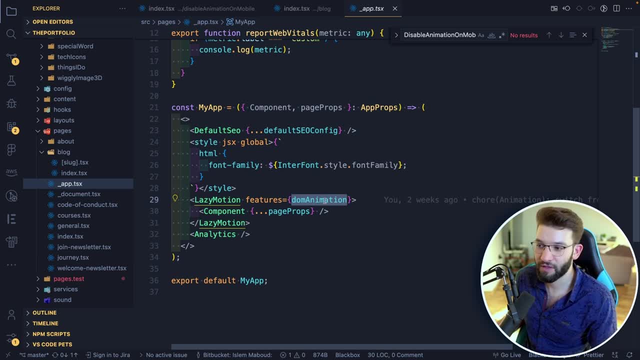 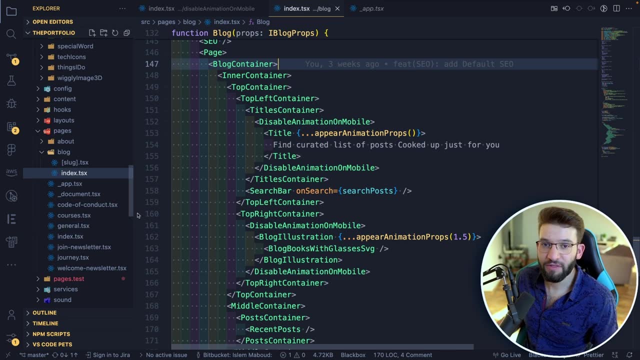 why import them? so it's better just to only import what you were basically using and that's basically what i'm using. i'm using only dom animation and just swap or basically just wrap my component in here and, for example, inside of the components later on when we try to do the actual animation, for example, if you go inside. 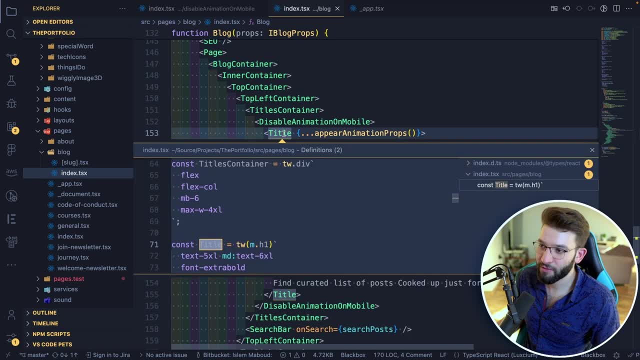 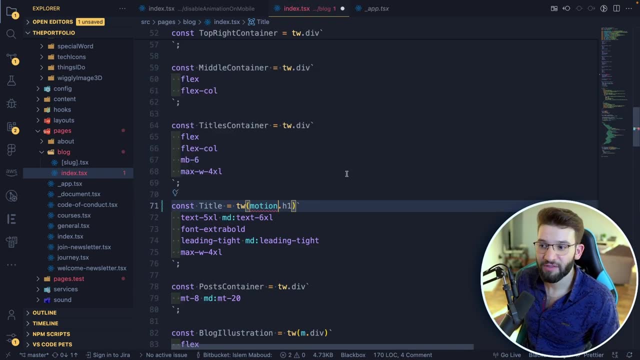 of the blog. so i go inside the blog in here, for example, the title. so i tried to look in the title. so the title in here actually uses the m instead of, like, the full motion one. we don't want to use that, so i want to only use the m in here to use the lazy loaded ones and only use those provided. 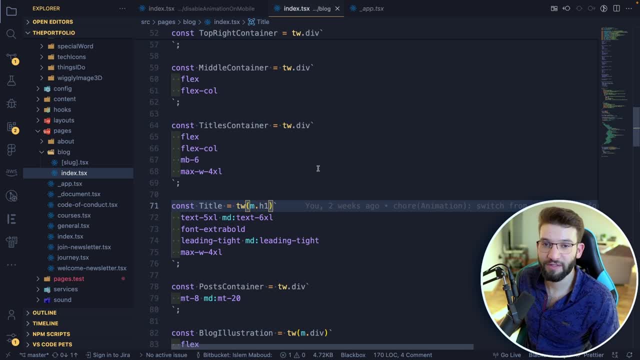 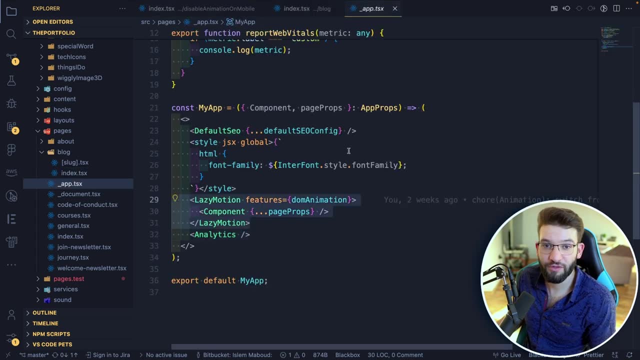 dom animations and, yes, this actually will help you cut the bundle size and quite a lot. and of course, the m in here is basically the same as the motion. it's only what you do in here just going to measure, or not? all right, so now for the sixth step that you must do for any website in 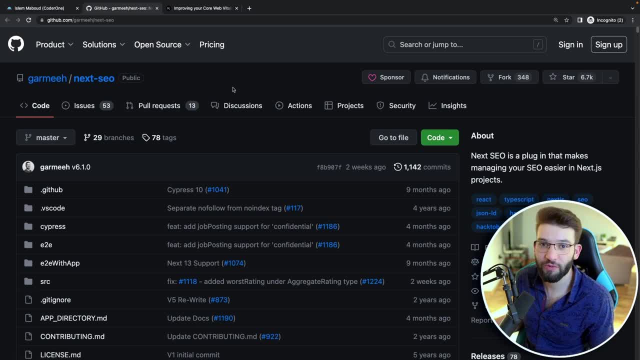 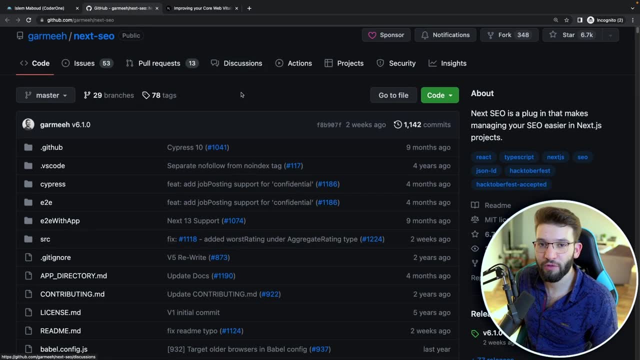 here and, of course, size. that actually need seo optimization, which most websites actually does. you want to use a really awesome package called the next total, so next seo in here is really awesome. library in here that works both for pages, so, which means the old connexiers like pages. 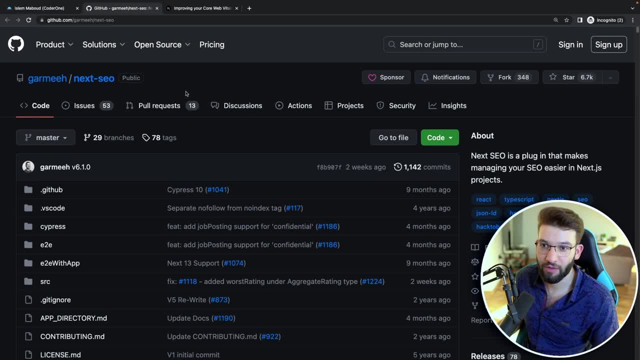 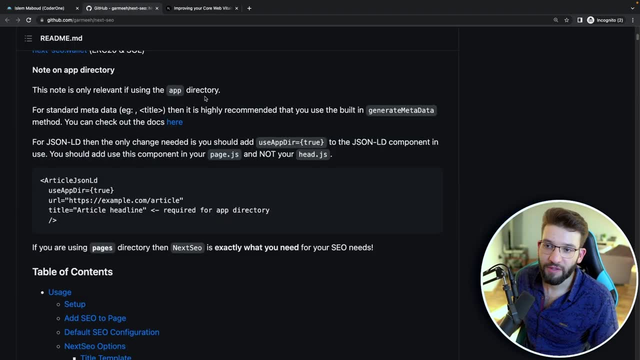 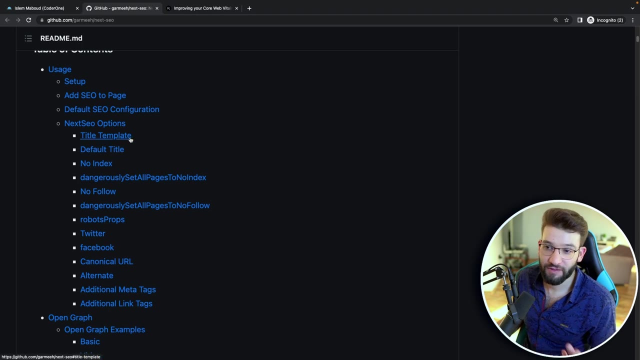 directory and routing system and the new up director for my current website. right now i'm using the pages and having fully migrated into the up just yet, but it works perfectly for both. so library allows you to basically add kind of like SEO for everything from open graph to a different stuff like changing the titles per page. basis Twitter. 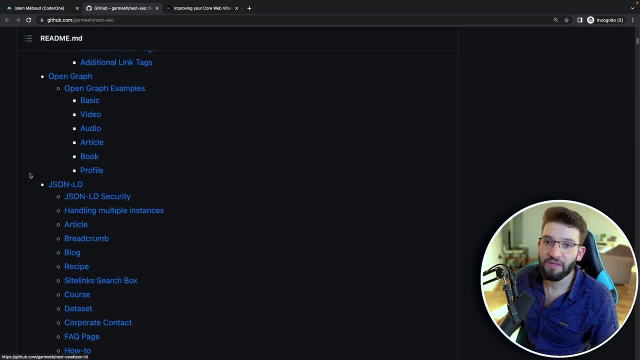 Facebook or canonical like URLs in here, or maybe you, Jason LD, in here to help optimize search optimization, For example, for Google search console, and using, like Jason LD in here, for different stuff, maybe using a blog or something. there are so many capabilities. 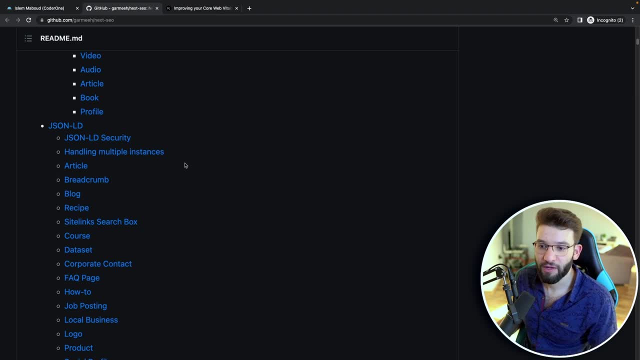 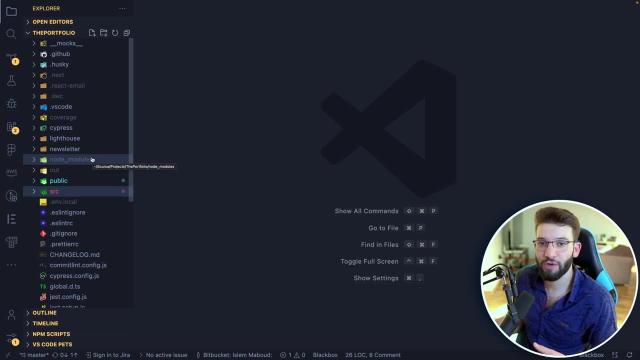 you can do using this really awesome library in a very, very simple way. So here I'm going to just going to show you what I actually needed for my projects, But of course, it depends on the type of project you have. You have a blog, you can do it this way. 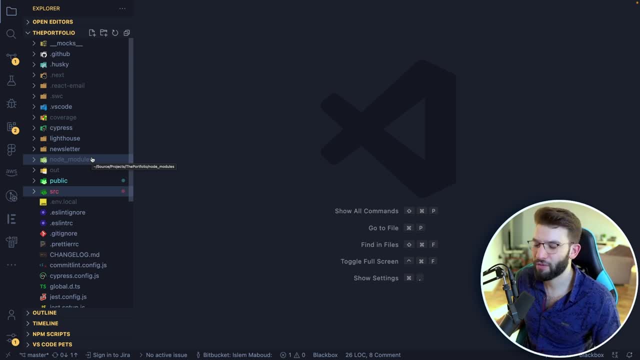 If you have articles or recipes, kind of like website, or any kind of website that needs SEO, it actually has a need for a specific kind of configuration. So that are going to be very, you know, quite a lot. So what I'm going to show you is actually the skeleton and what I did and what 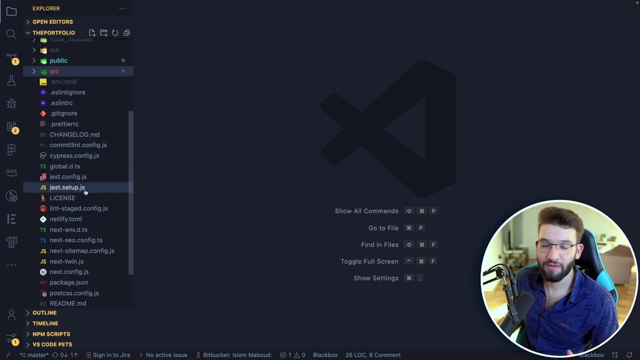 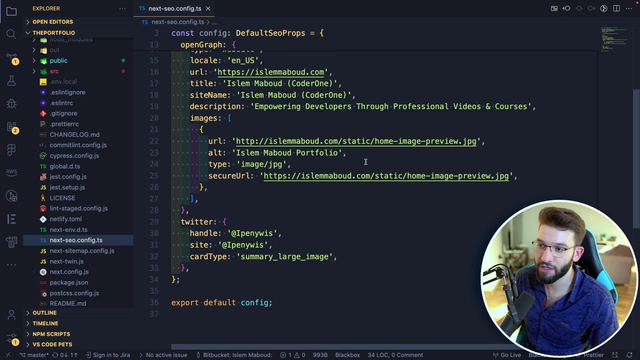 actually works for me and what made it super easy for me in terms of like developer experience. So first I installed the next SEO- as I said before, the really awesome package. Then I created this next-seoconfigtimescript, So this will tell next-seo that this is actually the default SEO configuration. 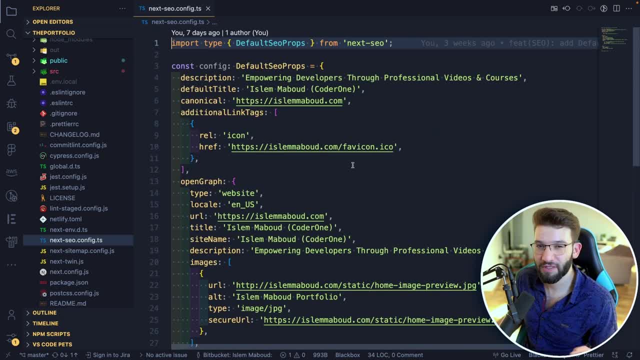 So, for like: for example, if the webpage doesn't have explicit or particular configuration for SEO, next-seo can fall back into this default one and can use it. So to start off in here is very simple. So all I'm providing here, for example description, is going to provide like: 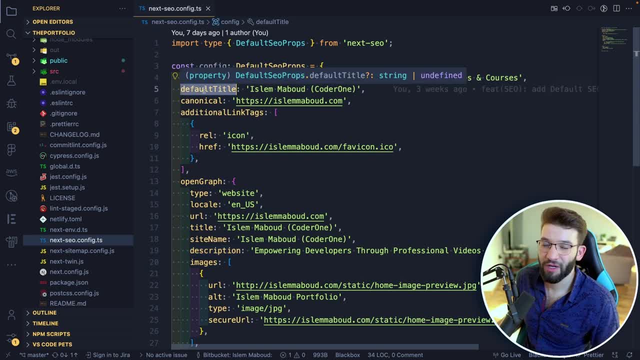 the meta tag description. a default title in here which is going to be applied by default if there's no title on other pages. uh, like you know, the the URL for the website in here. additional link tags in here: 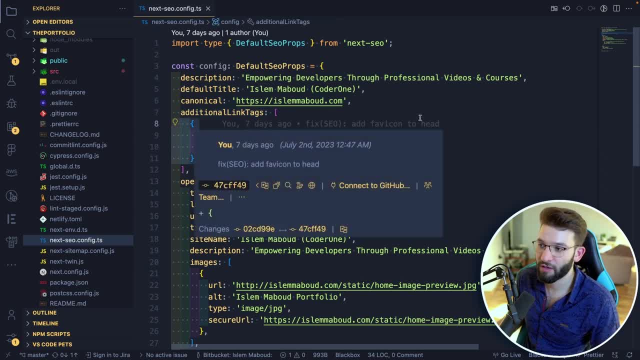 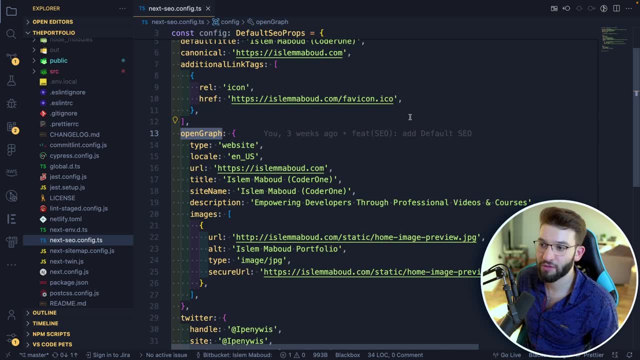 I'm using favicon in here, So it's actually. this is how you set the favicon And when it comes to open graphs, or open graphs basically used by social media like LinkedIn or Facebook or Twitter, to basically, when people share your website or content, tells you exactly what you want to do, for example. 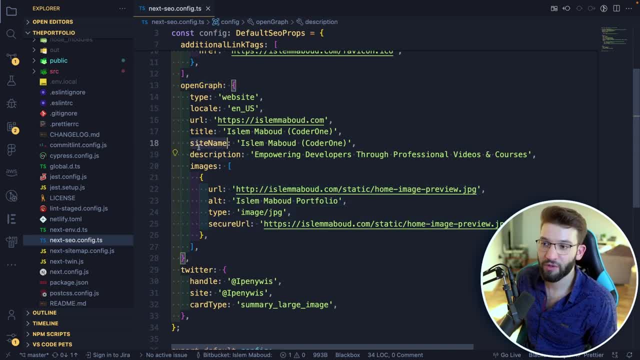 what image you want to display on the preview, what is the description going to put, what is the site name, title and stuff like that. So we want to make sure you put those correctly, and as well as the Twitter in here, which is like one. 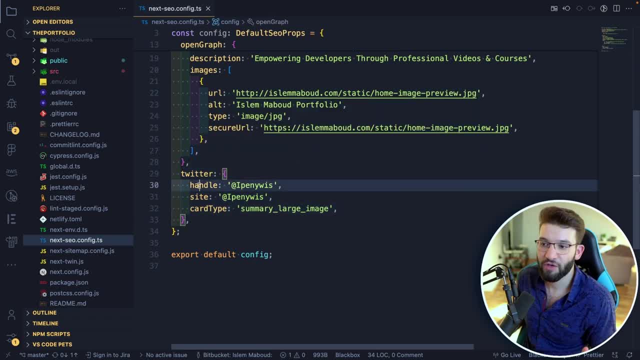 People share your stuff. You want to link them to an author and stuff like that, So you can tell: oh, this is the handle of the author. For example, this is my Twitter handle. Uh, this is the side of the author. maybe the card type in here like how: 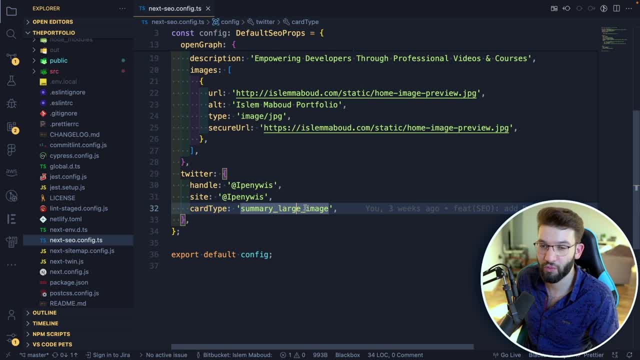 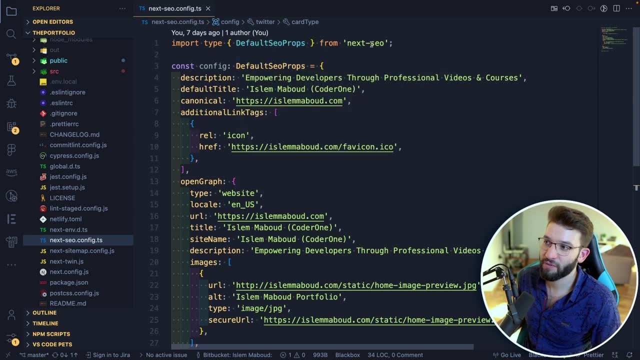 you want to show it when somebody tries to share it on Twitter or tweet about it. So there's actually a bunch of bunch of possibilities and using this really awesome like default SEO prompts in here is actually going to be using from the next SEO in here just makes it a lot easier. 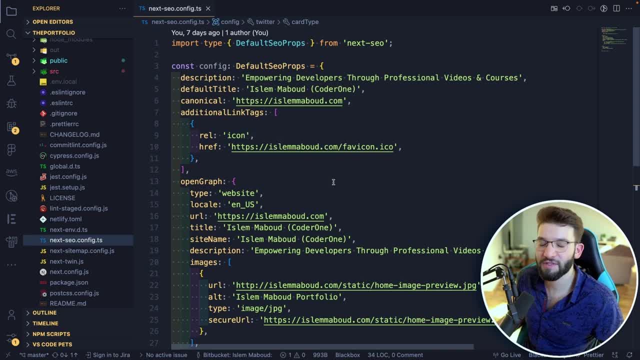 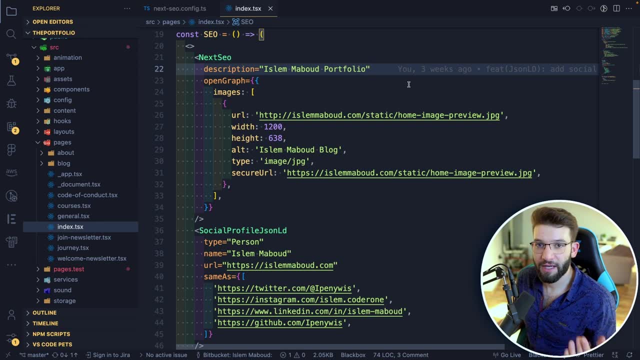 So instead of going through and actually putting the link mirror inside of the head every single time using it this way- quite simple. now the next thing I do in here is actually go into every single page that needs some custom stuff or like custom SEO configuration. 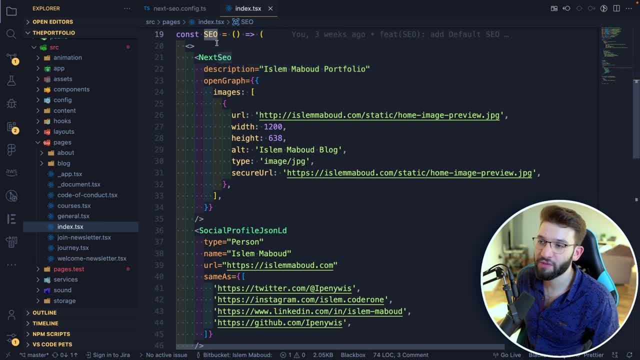 in here and actually overwrite that. So what I do? I go to SEO in here and create like a component on every single page in here, for example, the index or the landing page in here. I use the next SEO component and try to put all those as props. 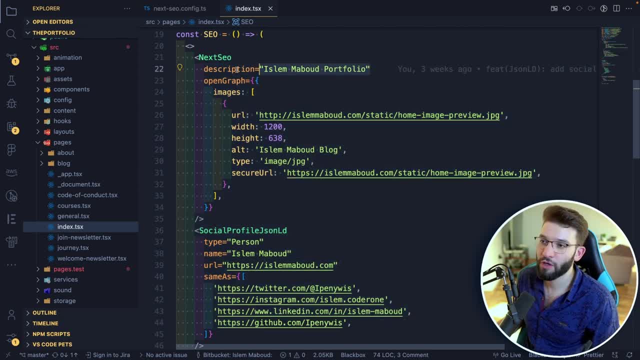 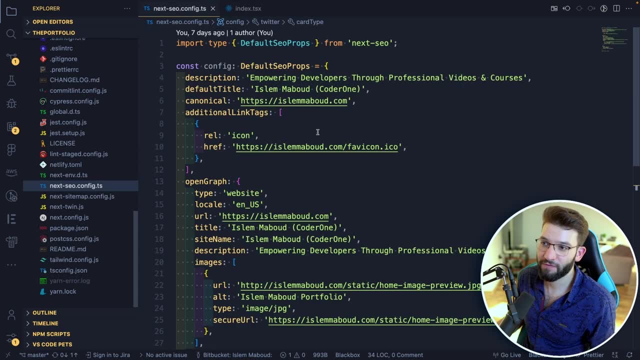 So I put the description for example: oh it's like my board in here portfolio and just a quick notice in here, So whatever, like you kind of like ignore from this. next SEO is going to Like bring it from the default category. 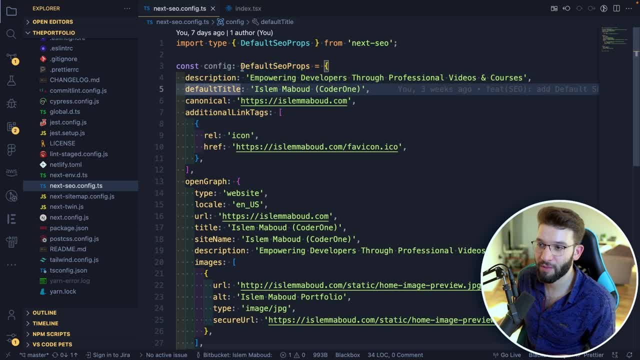 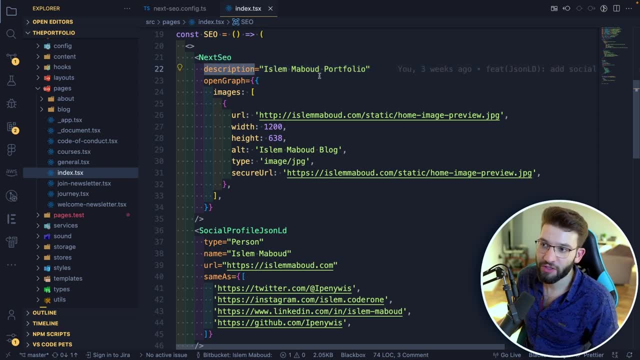 So if you have like a default one and you only want to override a couple of block parameters or options, you can only just overwrite those in here. It's going to fall back to the default for the missing ones. So for example, in here I'm only changing the description. 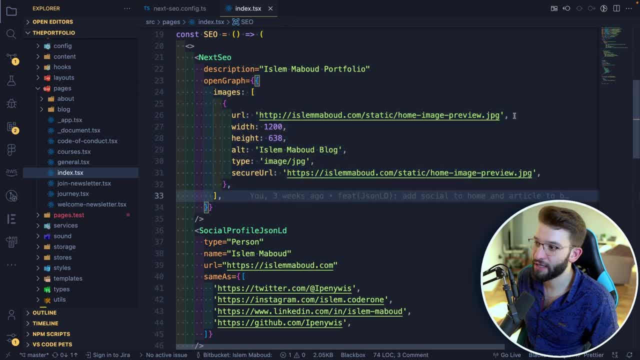 I'm not changing the title and I'm changing the open graph images And so I'm setting specific different image in here with like specific width and height, and you also want to set the all to type. so it's, it's huge thing in here. 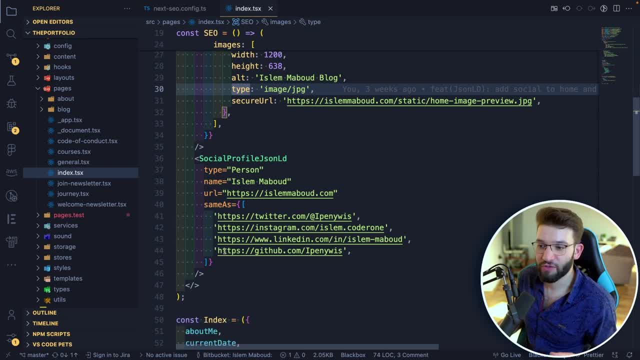 Also, what works for me really, really well is actually is the JSON LD, because JSON LD in here is like a specific format Me By Google to help their- you know, Google search kind of like engine or robots to basically scroll your website quite easier and actually have a better kind of preview. 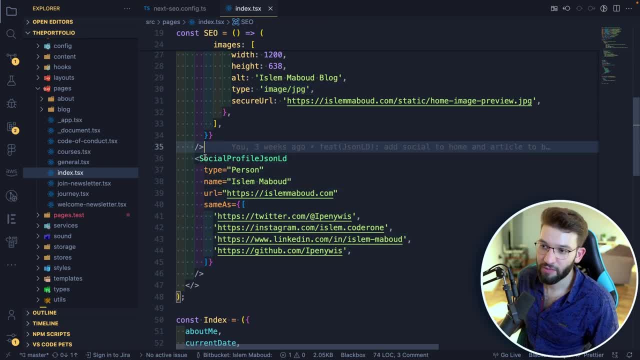 on the on the Google search results, So this one actually works as well. So I'm using here, for example, the social profile, Jason, which is to tell it how you want to like. what is a profile? Where's my profile? 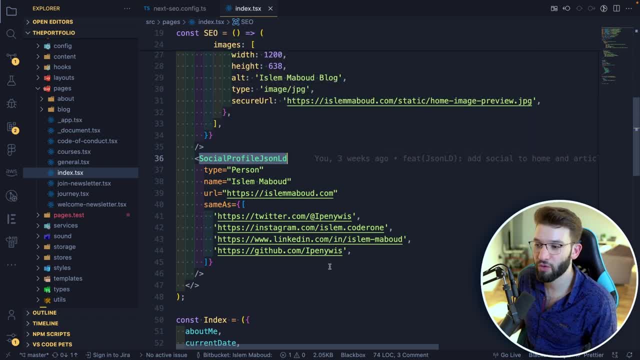 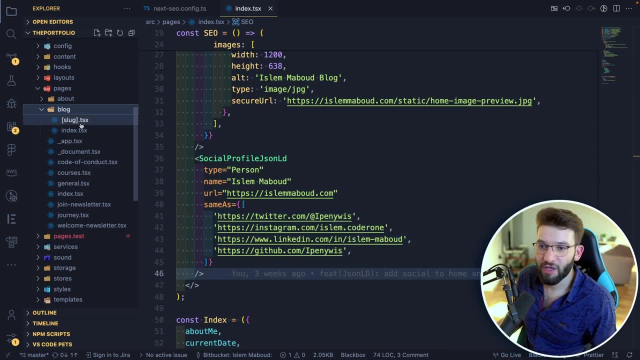 So if somebody actually shares that when it tries to do some quick search on Google it's going to display potentially my profile from one of these kind of like related, um you know, social platforms And it actually keeps Going. So if you go inside of the blog in here you have, and it actually keeps going. 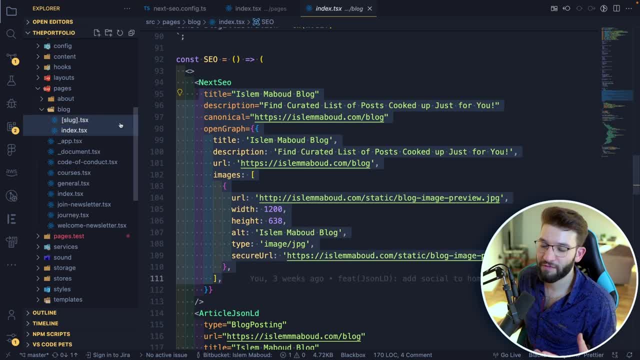 So, for example, if you go inside of the blog in here, you have different configuration for that. If you go to I don't know about there, you have different configuration and keeps going, and keeps going. So there's so many things in here. 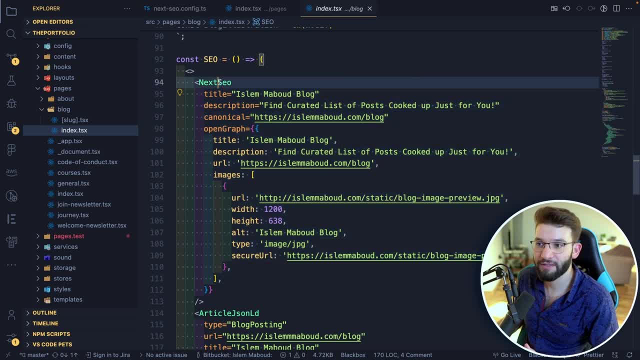 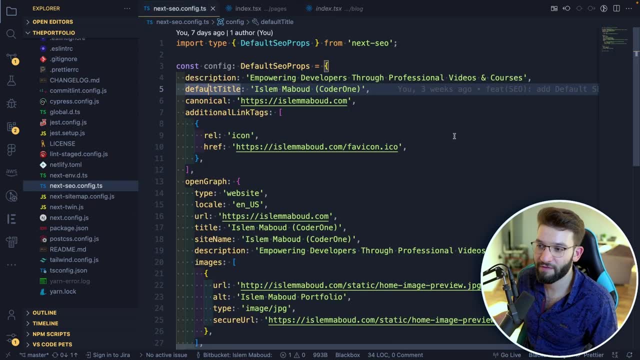 So there's actually- I'm doing it on every single page in here. I'm actually overriding the next SEO with different configurations and stuff And I'm having a default one in here, So for fullback for pages that you know doesn't have that or something. 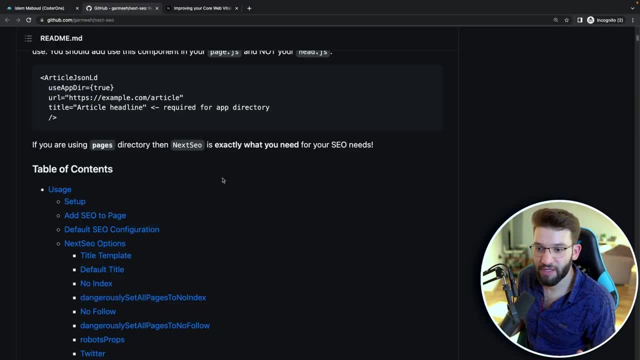 I'm just using this as a default, I think, the best way to approach SEO in here, because it has so many things in here I can't cover it in one single video, So going through like next SEO in here. So try to access this read me page of this library in here and get home and 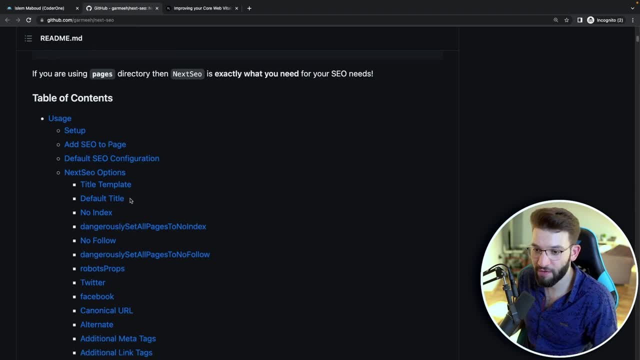 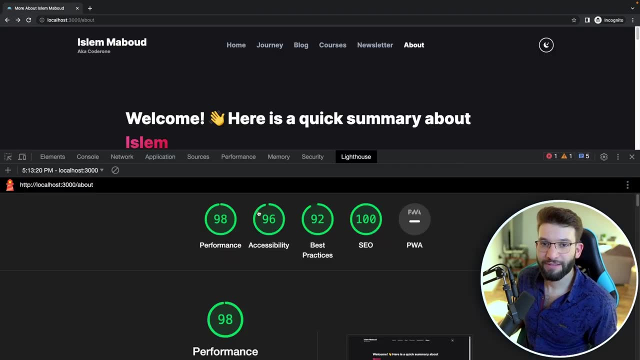 try to read through the- read me in here- the table of contents and actually go through every single one of these, you will better understand exactly what they do and if you ever need them for your website or not. if you try to quickly test the lighthouse or run the lighthouse score again, you're going to find a lot. 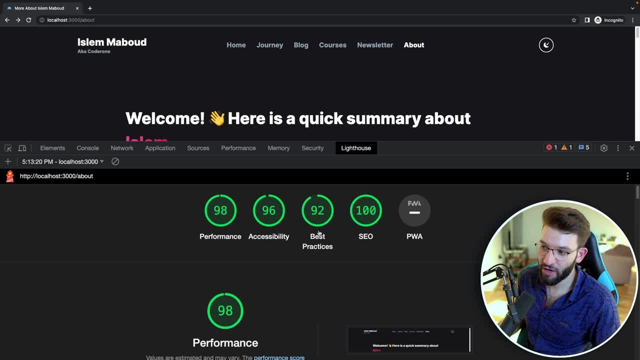 of differences in performance, accessibility, maybe also best practices. in here, and particularly SEO, is like a hundred percent. If you make sure that you apply all the SEO best practice and use next as SEO properly and have all the parameters covered up, you will get hundreds score on SEO. 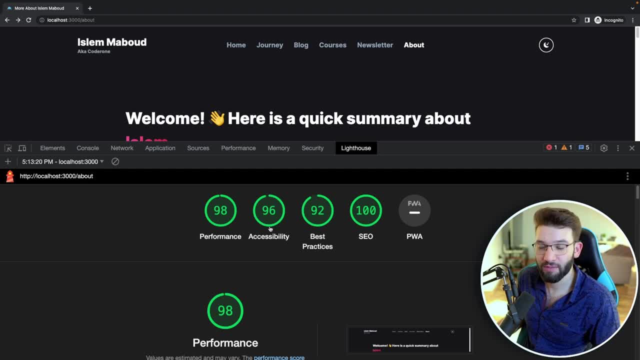 And when I talk about SEO, there's actually some stuff that are also related to accessibility. So fixing SEO will fix a lot of accessibility issues as well. Now for accessibility particularly, you can actually improve that as well. So there's actually some stuff from teeny tiny stuff that actually can. 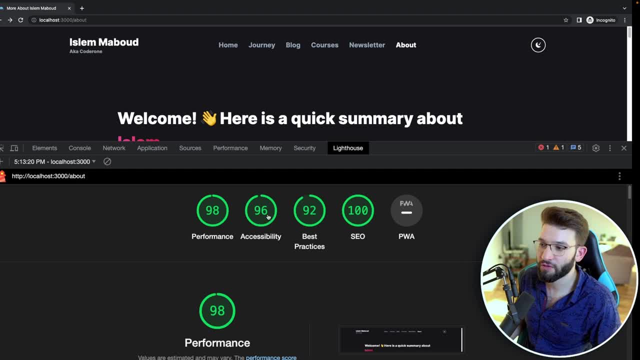 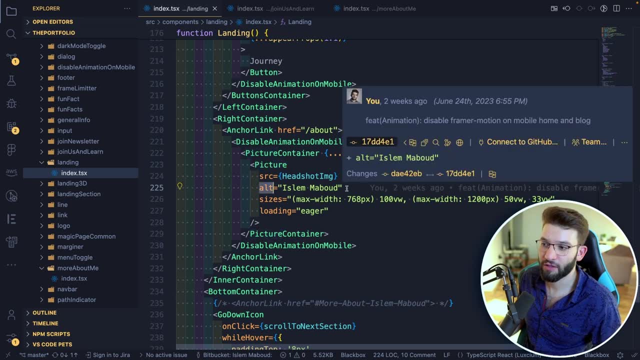 improve the accessibility in here and improve your score overall. So, for example, in here, when it comes to that, for example for pictures, what you want to make sure you do always is actually provide an Alt in here. So Alt R2B is going to give a lot, if like a lot of a advantage in the 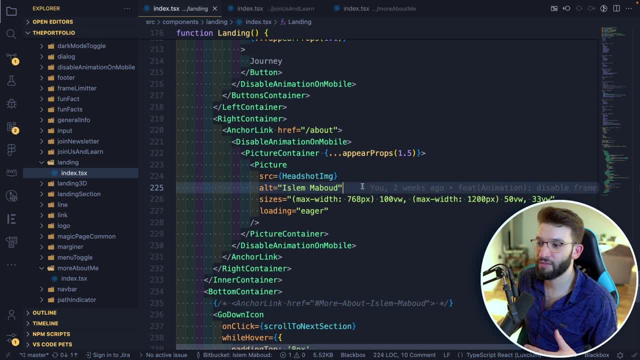 accessibility score in here, because it's going to provide, you know, to search engines and, you know, to accessibility settings in general, like what the image is for people who, like you know, can't see the image for some reason. you know what I mean. 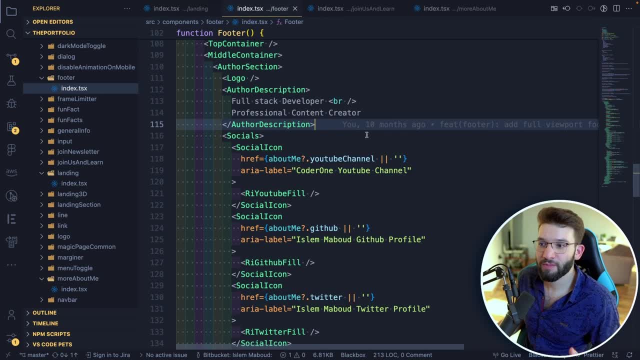 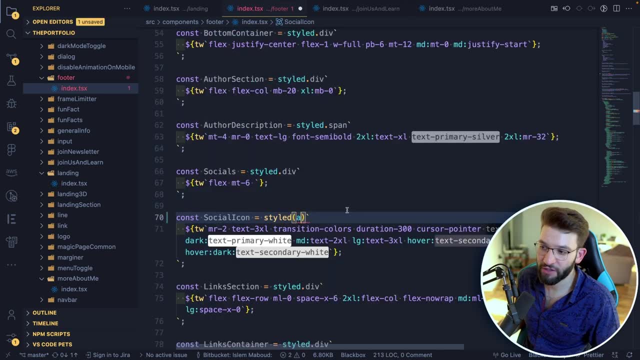 So this actually can work quite a lot, As well as when it comes to links, for example, when you've got this social icon, which is on itself an anchor link. So an anchor link here which is basically Just like an H or a link in here, just that's what it is. 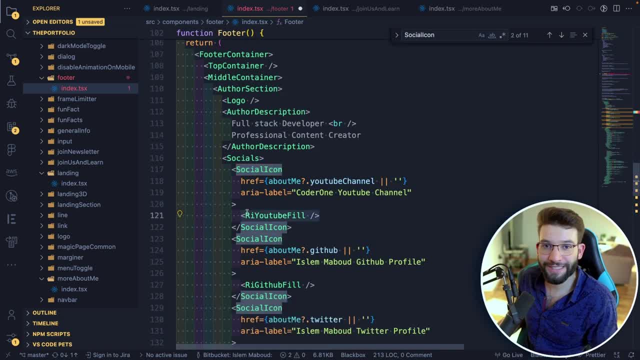 So for social icon in here, have those social icons where there's no text inside of it, just basically have the parents and the child in here is just simply an SVG icon. So this will actually break your accessibility. So to basically fix it, because accessibility needs to always make sure you have some. 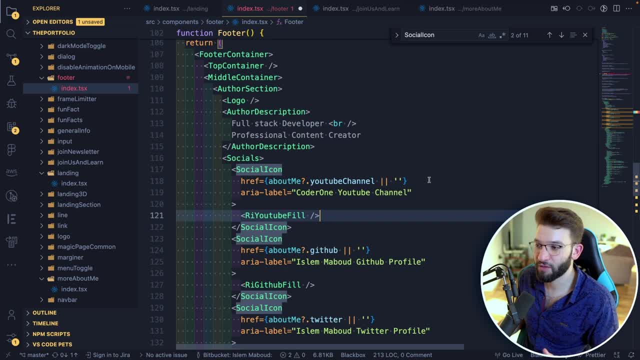 text in here to display for people that actually can't see those particularly So what you can basically do is actually replace it with this area label kind of attribute, and every label in here is going to act as a, you know, like a replacement text for people that basically can't see that kind of image. 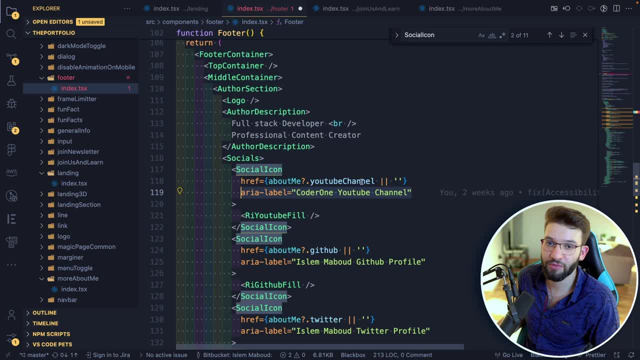 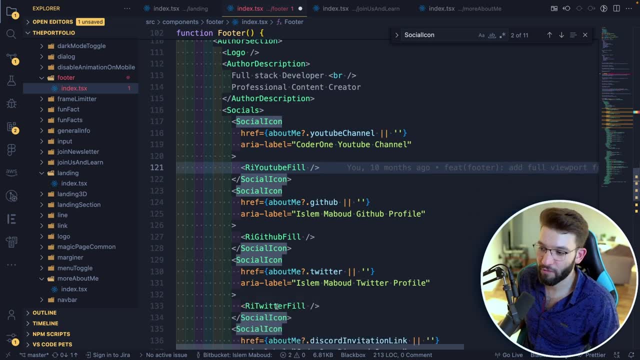 in here is going to like see this, this area label kind of thing which kind of represents exactly what this social icon is about. So, for example, he's like code one YouTube channel or maybe some I would get a profile. 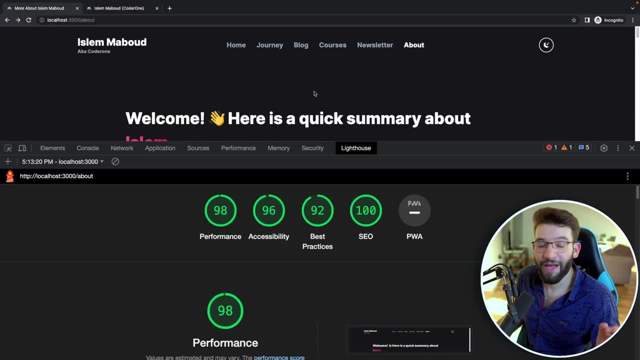 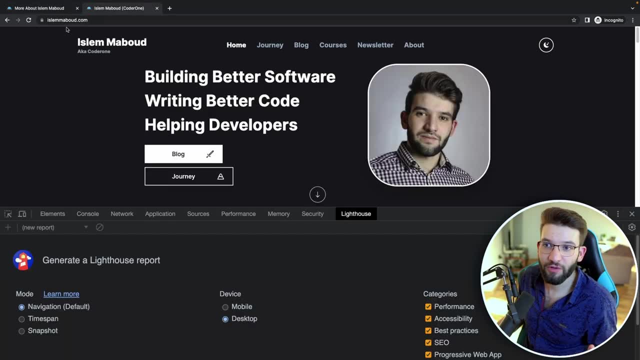 So it basically just a quick description of what this one is, And there you go, And this should actually give you a really good score when it comes to, you know, lighthouse score in here, Every example, if you want to test this with a deployed one, so like: